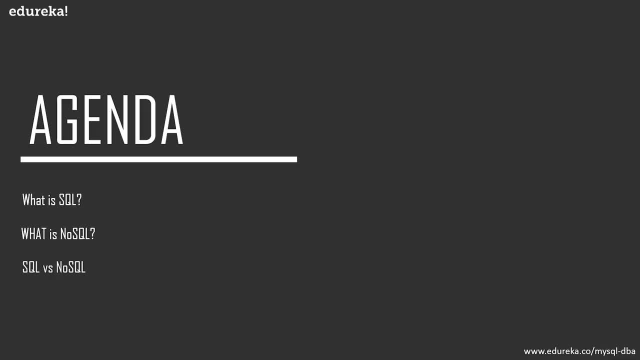 I'll introduce you to one of the most popular databases in today's Market, that is, my sequel and MongoDB- and finally, will end the session by comparing these databases too. So I hope the agenda is clear to you guys. All right, so that's great. 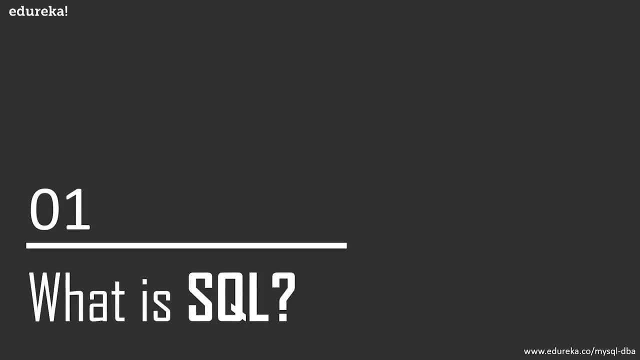 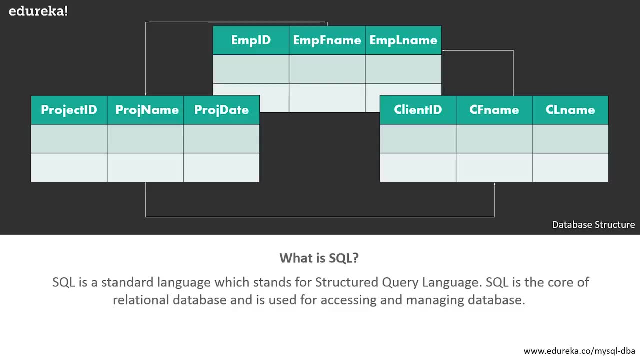 So let's get started with this session by understanding what is sequel. sequel is a standard language which stands for structured query language. sequel is the core of relational database and is used for accessing and managing the database, So this language basically helps you to retrieve the data. 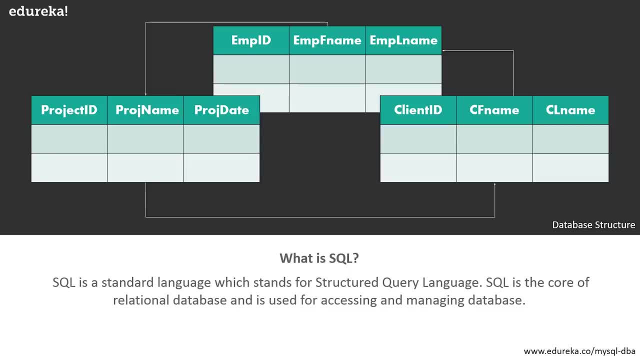 from a database whose structure is completely made of tables with rows and columns, and these tables are interlinked with each other with specific values which can be retrieved from these tables with the help of queries. as it is So, as you can see on the screen over here, 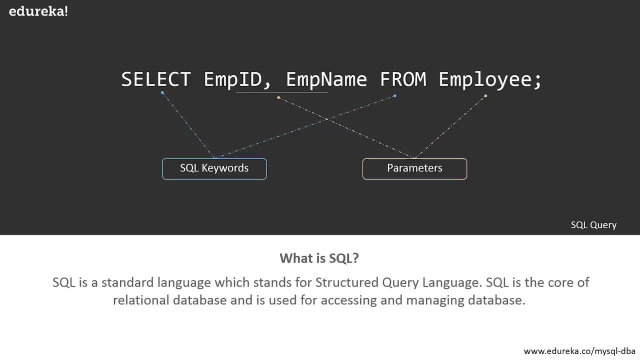 we're trying to retrieve the employee ID and the employee first name from the employee table. So if you observe the query, you can clearly see that you know the query has sequel, syntax or keywords, and also has few parameters which indicate what data has to be retrieved. 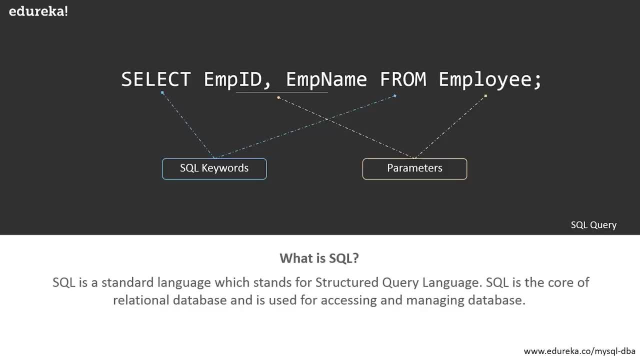 So if you observe the query, you can clearly see that the query has sequel syntax keywords. So basically, the select and the from are the sequel syntax keywords and the employee ID, employee name and the employee are few parameters which indicate what data has to be retrieved from where. 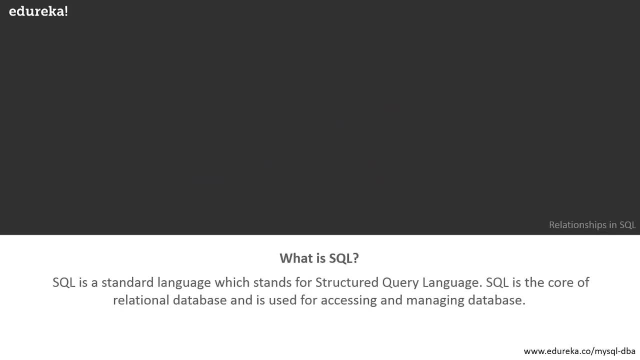 so I hope this point is clear now. not only this, but sequel also enables you to maintain relationships between tables. Now these could be either one-to-one relationship, one-to-many relationship, many-to-many relationship or self-referencing relationship. Now, one-to-one relationship is 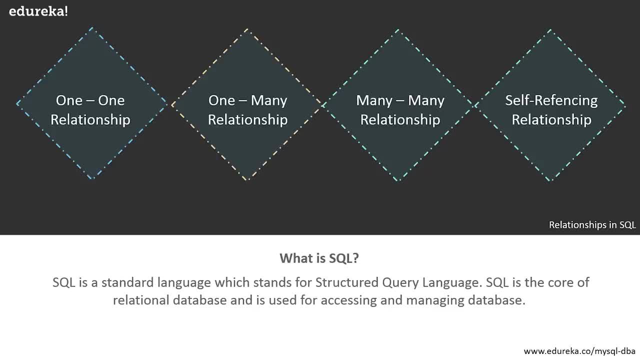 when a single row in a table is related to a single row in table B. So when I say single row, I basically mean record. so each record and table a is related to a single unique record in table B. Now, similarly, one-to-many relationship is: 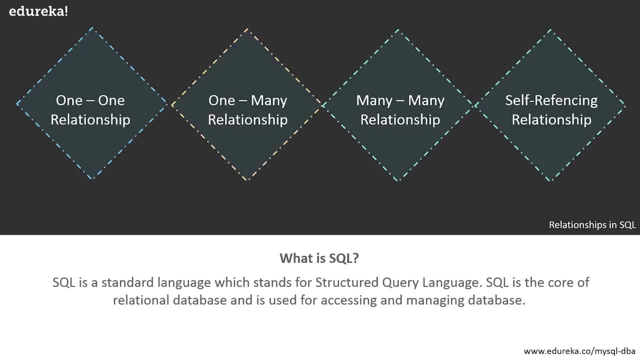 when a single row in table A is related to many rows in table B. by that I mean that you know, one unique record from table A can be related to n number of records in table B. now, similarly, coming to the many-to-many relationship: the many-to-many relationship. 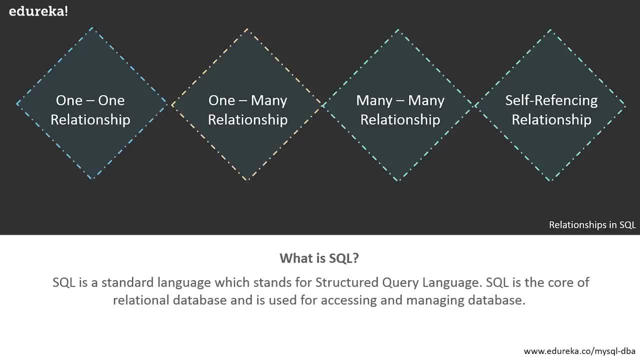 is when many rows in table A can be related to many rows in table B. And finally, the self-referencing relationship is when records in table A are related to the same table itself. So that's when we use a self-referencing relationship. 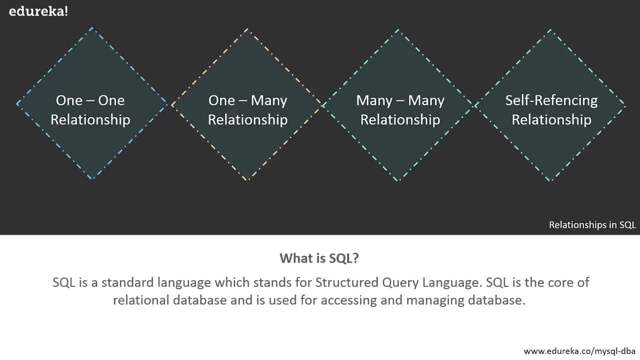 So, guys, these were the various types of relationships also available in sequel. Now, if I have to just summarize sequel for you, then sequel is a language which helps you to retrieve and manipulate data from well-structured databases with the help of queries and commands such as insert, update and delete. 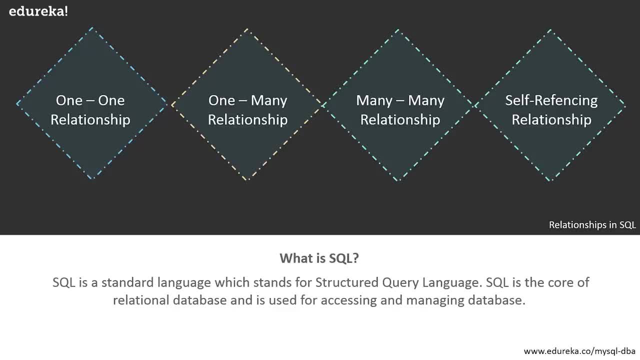 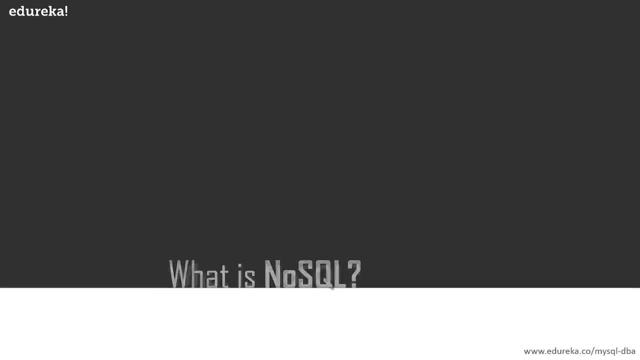 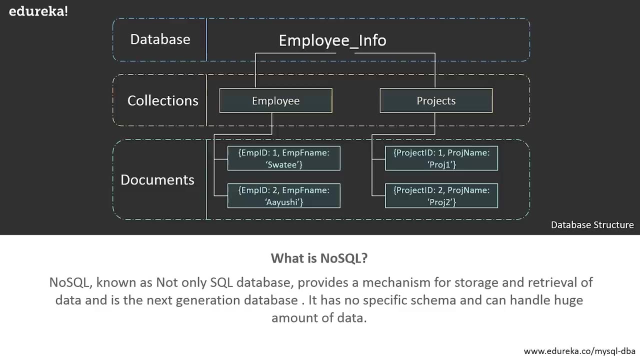 and also maintain the relationships present between the tables in a database. So, guys, I hope you've understood what sequel is. now Let's just understand what is no sequel. no sequel, or most commonly known as not only sequel, database provides a mechanism for storage and retrieval of data. 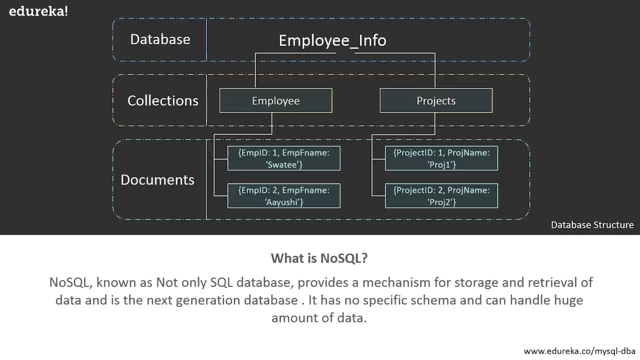 and is the next generation database. this kind of database has no specific schema and does not have tables with rows and columns storing data values, but can definitely handle large amount of data. So, if you consider the example on the screen, we have an employee database which has two collections. 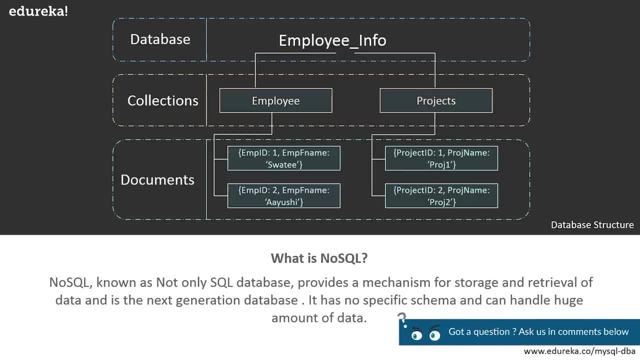 that is, the employee and the projects collection. now, each of these collections have documents, which are basically the data values. So if you just want to understand these terms, then you can just consider the collections to be a tables and the documents to be your fields in the tables. 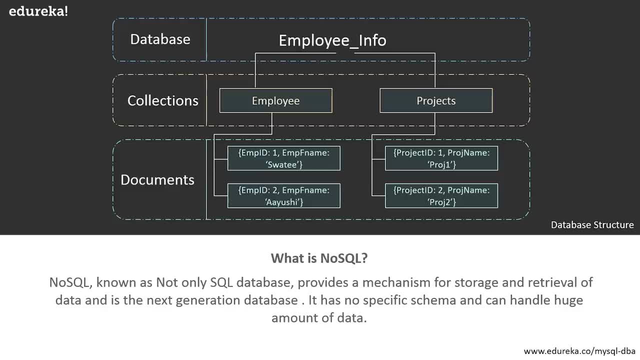 So if you compare a sequel database and a no sequel database, for example, let's just say we have an employee database where you know there's an employee table with around 10 columns, right, That is basically the 10 fields now in the no sequel database. 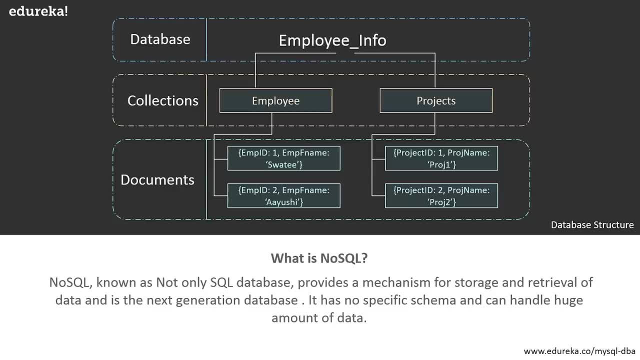 What will happen is the employee table itself will be taken as a collection, and each of these fields will be considered as documents. Now, the most interesting part of no sequel is that these kind of databases do not have to use the same schema for the presence of multiple documents in one collection. 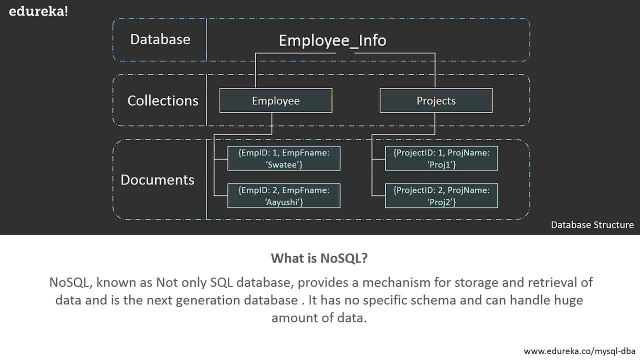 So, since no sequel has dynamic schema, that means that you know multiple documents can be present in a single collection and also each collection can have different documents. So you can have a document in the collection which has both employer ID and employee name, and also you can have a document 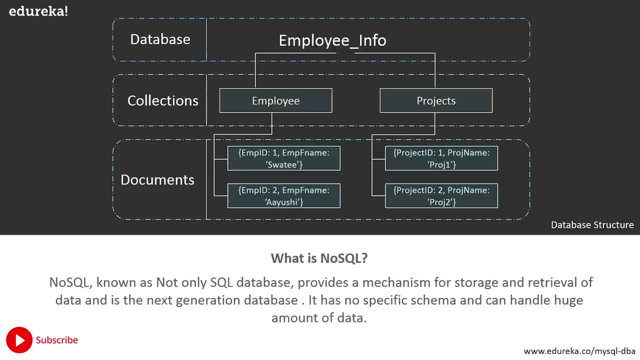 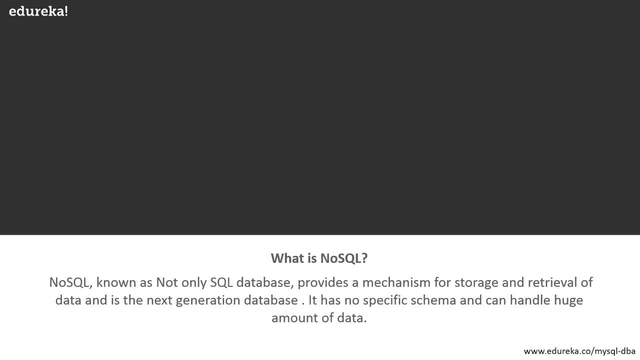 in the same collection which do not have the ID and just dose the name. So that's how, guys, you can play around with collections and documents in no sequel database. apart from this, Let me just also tell you that you know there is no specific query language present in no sequel. 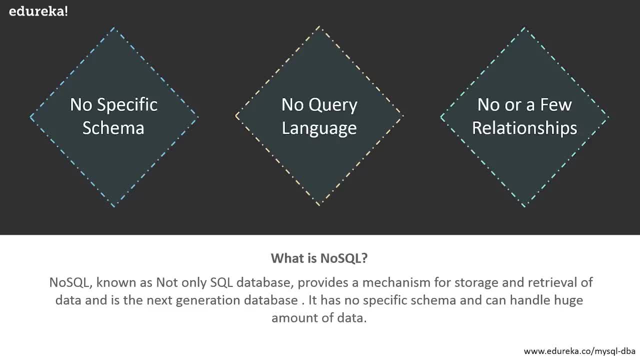 So, basically, the language that you use to retrieve data is completely infrastructure based. That is basically how you store your data and where you store your data. Lastly, there are no or very few relationships present in a no sequel database, As you do not have a predefined schema. 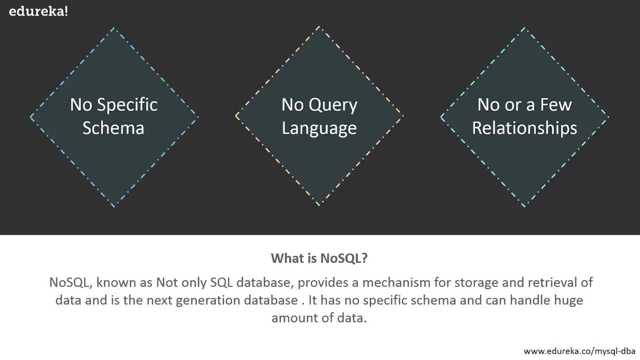 but you do have a dynamic schema in which we can put all the required information in a collection. right, when you have a dynamic schema and you have the option of putting all the required information in a single collection and the collection can differ in the same schema itself. 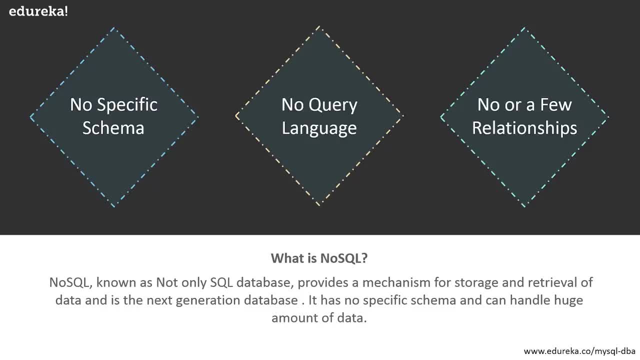 You actually do not need any relationships to be present, right? So that's how, guys. no sequel does not have, or has very few relationships. So, guys, if I just have to summarize no sequel for you, then no sequel is a type of database which do not have a predefined schema, a query language. 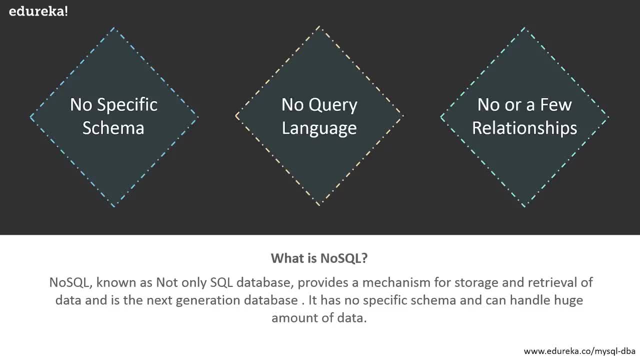 and has no tables. It follows a method of storing data in a dynamic schema with less or no relationships, and can handle humongous amount of data. So now that you know what sequel is and what no sequel is, Let's now see how these databases stand against each other. 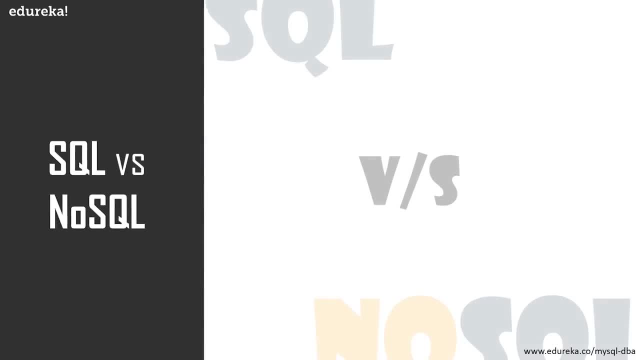 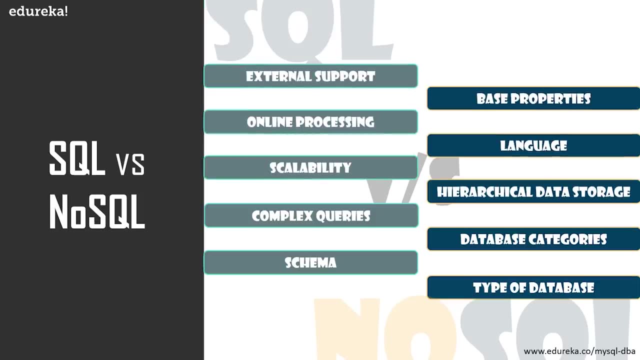 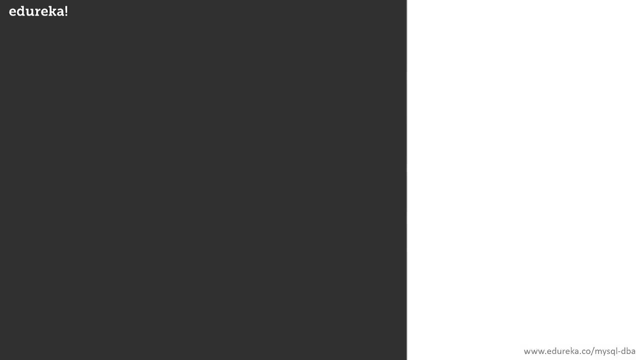 So, in the space of, will be comparing both these databases based on the ground, such as the type of database, schema, database categories, complex queries, hierarchical data storage, scalability, language, online processing based properties and external support. Let's get into the detail with the first comparison factor, that is, type of database. 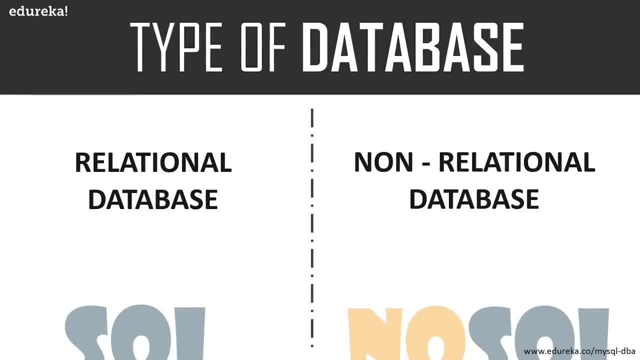 Now, when we compare these databases based on this factor, let me just tell you that you know, sequel is essentially called a relational database and it organizes structured data fields into defined columns. So database can have n number of tables and each table can have m number of columns. 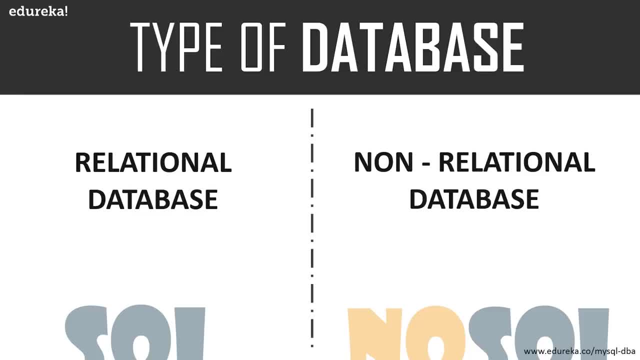 with the data stored in it. Each table can be related to the other tables also, right? So if you have around 10 tables, then those 10 tables can have around two to three columns, or you can say more than that columns in each table. 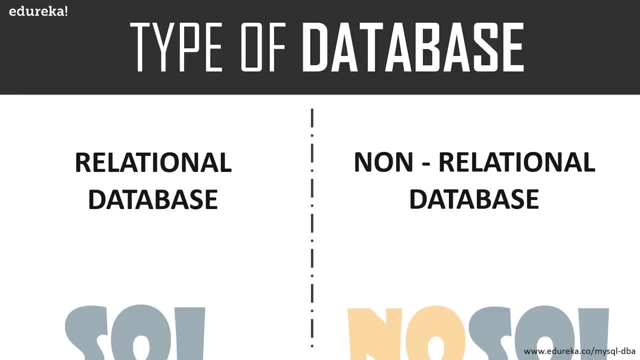 and all these 10 tables can be related to each other. coming to no sequel. No sequel is a non-relational database which provides a mechanism for storage and retrieval of data. in the no sequel database, data is modeled in the form of collections and hence it tries to avoid relations. 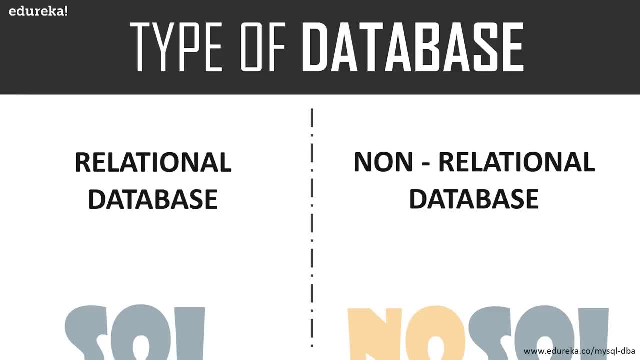 as I just explained you before. so, guys, if you have to compare these databases based on this factor, then sequel is essentially a relational database and no sequel is a non-relational database or a distributed database. next We'll be comparing these databases based on the schema. 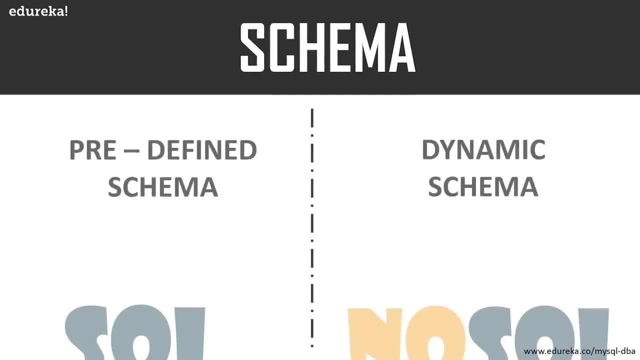 but comparing these databases based on this factor, Let me tell you that sequel needs a predefined schema for structured data. So before you start using sequel to extract and manipulate data, you need to make sure that you know your data is predefined in the form of tables coming to no sequel. 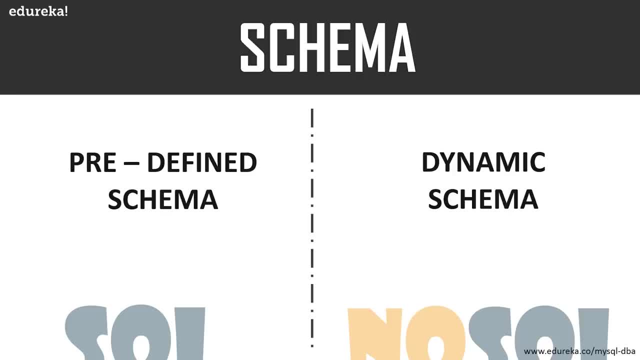 Well, no sequel databases have a dynamic schema for unstructured data. So if you're using the no sequel database, then there is no predefined schema present and the complete schema of your data completely depends on how you wish to store the data, that is, which feels. 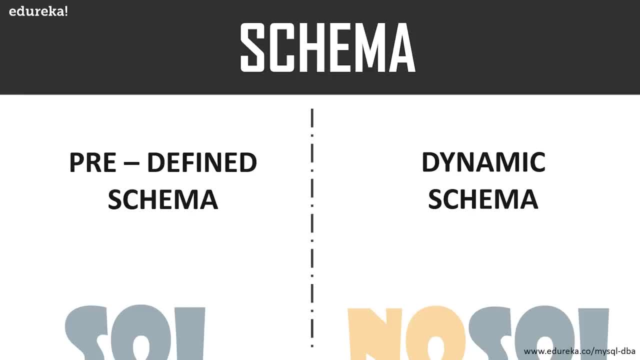 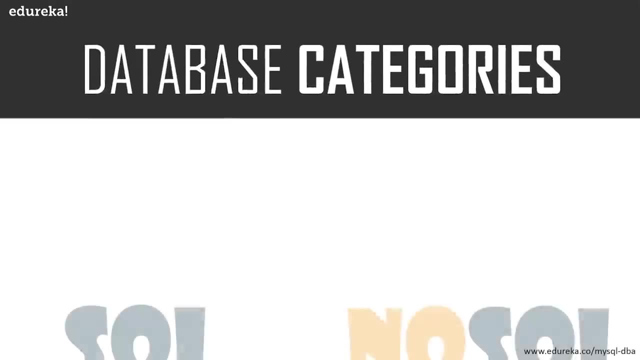 that is basically which documents that you wish to store in which collections and how you wish to store them. So, guys, that was about schema. the sequel has a predefined schema and the no sequel has a dynamic schema. now moving on to the next parameter, which is database categories. now sequel database. 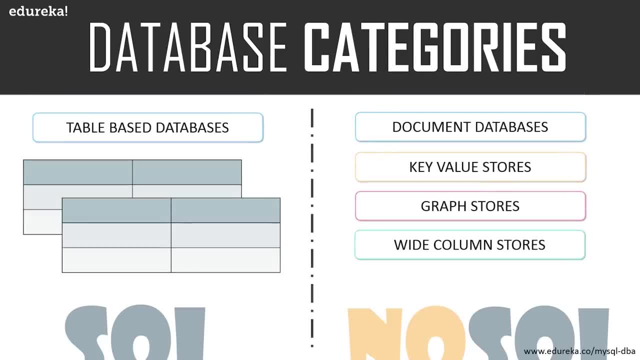 databases are basically the table based databases. So, as I explained in the previous factors, the sequel databases can have n number of tables related to each other and each table can have M number of rows and columns storing data in each cell of the data. Now, similarly, if we talk about the no sequel databases, 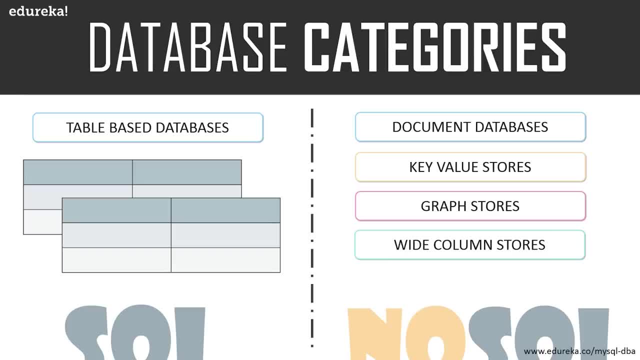 the no sequel databases have mainly four categories of databases, that is, document database, the key value stores to craft stores and the white column stores. coming to the document database Now, this kind of database pairs each key with a complex data structure known as a document. it can contain many different key value pairs. 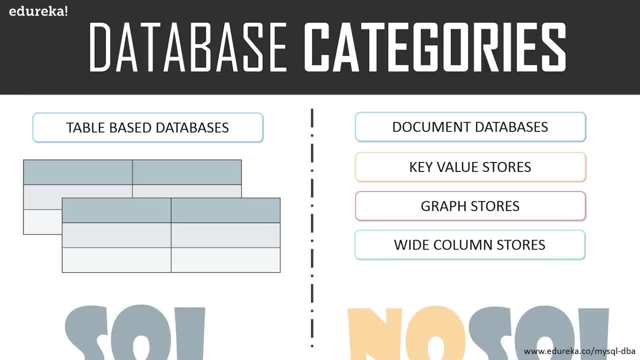 or the key error pairs or even the nested documents. coming to the key value stores, These are the simplest form of no sequel database, So every single item in the database is stored as an attribute name or a key, together with its value. now coming to the craft stores. 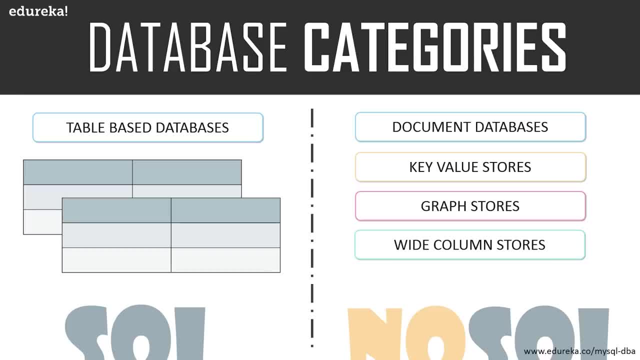 The craft stores are basically used to store the information about networks such as the social connections that the craft stores mainly include, the neo4j and the hypergraph TV. coming to the last kind of database category of no sequel, that is, the white column stores, the white column stores, such as Cassandra, 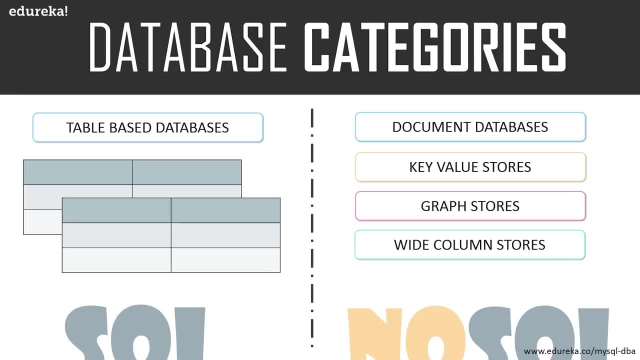 and H ways are optimized for queries over large data sets and stores columns of data together instead of rows. So, guys, these were mainly the four categories of no sequel database, that is, the document database, the key value stores, the craft stores and the white column stores. now, this might have given idea. 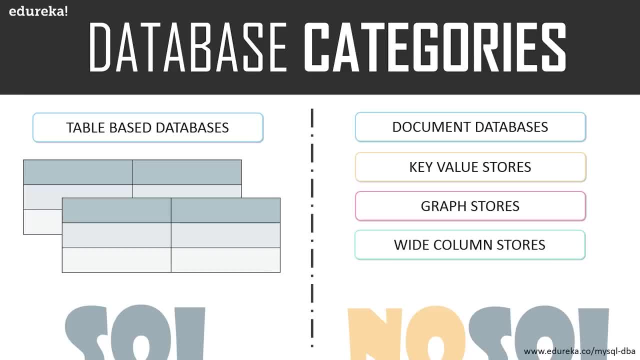 of you know, the sequel databases basically represent data in the form of tables which consists of n rows of data, Whereas the no sequel databases are the collection of key value pairs, documents, graph databases or white column stores which do not have a standard schema definitions. 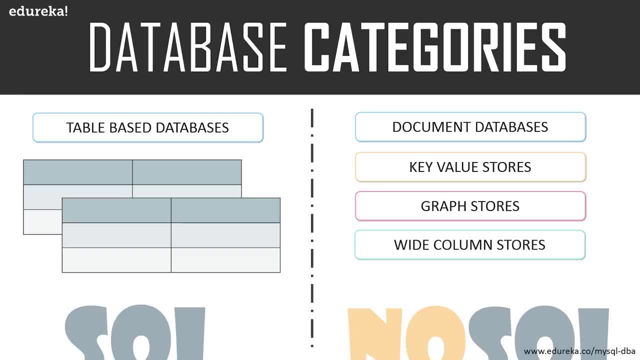 which it needs to stick to. so, guys, this was the main difference between sequel and no sequel. that sequel is basically the table based databases with a predefined schema, and the no sequel databases mainly have different categories of databases with a dynamic schema. So I hope I'm clear with this point. next, 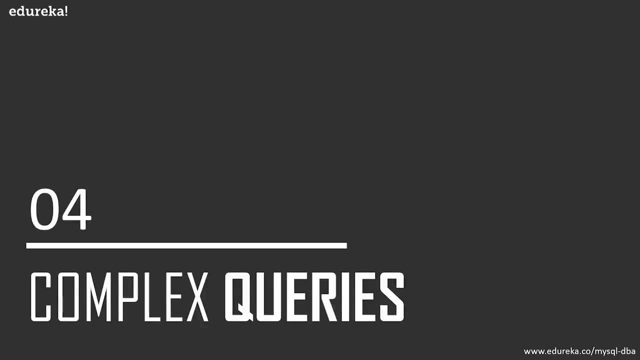 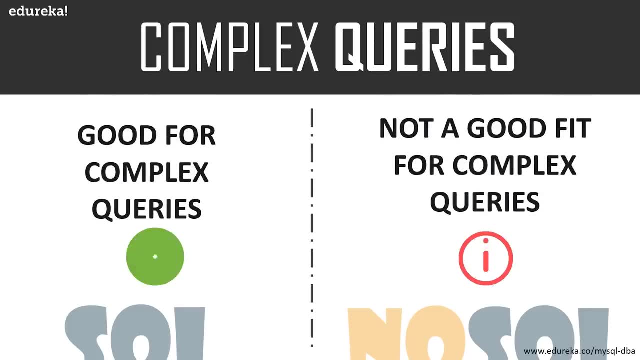 Let's discuss how these databases fit for complex Queries. now, when we talk about complex queries, let me just tell you that in a sequel is a good fit for complex query environment, as the schema in sequel databases is structured and has proper tables. So even if you wish to apply nested queries, 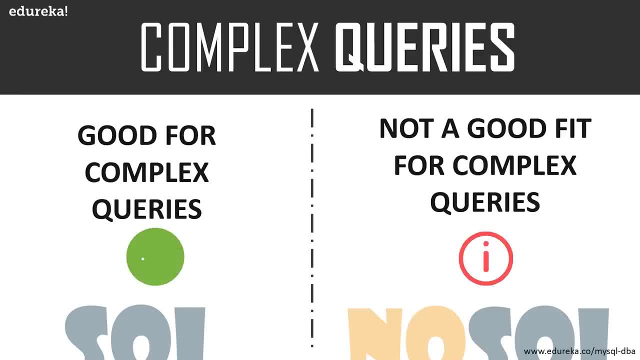 with many sub queries inside the outer query. you can easily do by using the proper table and column names and you can retrieve the required data. coming to the no sequel databases, The no sequel databases are not a good fit for complex queries as they don't have standard interfaces. 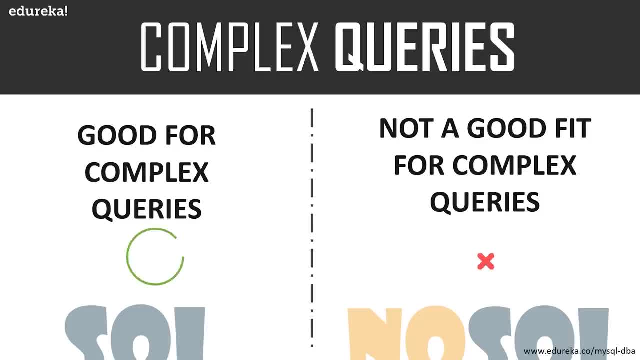 to perform complex queries and the queries themselves in no sequel are not as powerful as the sequel query language. So this is basically because you know they're not written in a specific language and the language in which they are written is completely based on the database infrastructure. 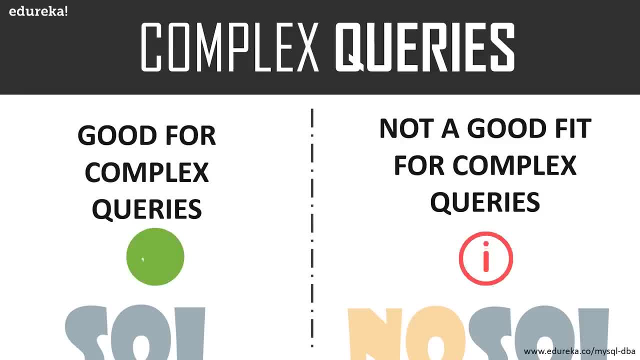 You can see the schema. So if you have to compare how these databases fit for complex queries, then let me tell you that sequel is a better fit for complex queries when compared to no sequel. now moving on to the next factor of comparison, that is, hierarchical data storage. 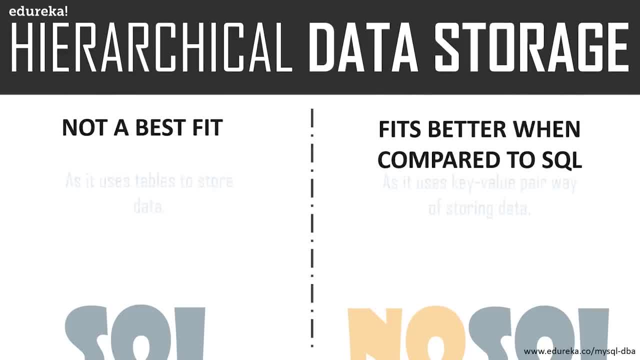 Now, when we compare the databases based on this factor, let me tell you that the sequel databases are not best fit for hierarchical data storage. now, this is because, as the number of tables increase, the complexity of relating them to each other also keeps increasing. now, in such a scenario, 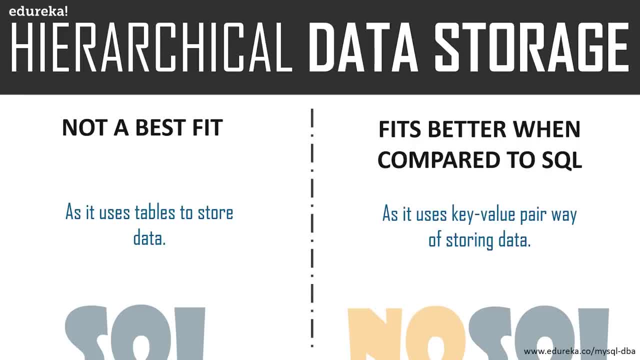 you cannot relate humongous amount of tables with n number of columns to each other, right, but coming to no sequel database, the no sequel database fits better for hierarchical data storage as it follows the key value pair way of storing data similar to the JSON data. 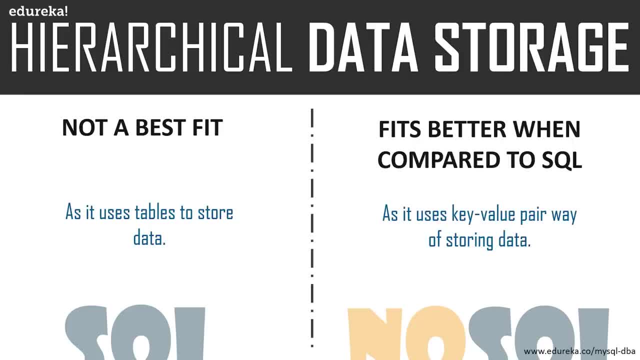 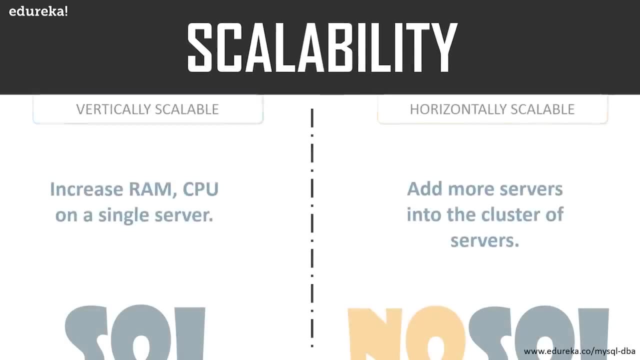 Now, no. sequel databases are also highly preferred for large data sets when compared to the sequel database, and one such example is HBase. So basically, HBase is used for this purpose. next point of comparison will be scalability. now, sequel databases are vertically scalable. You can load, balance this database. 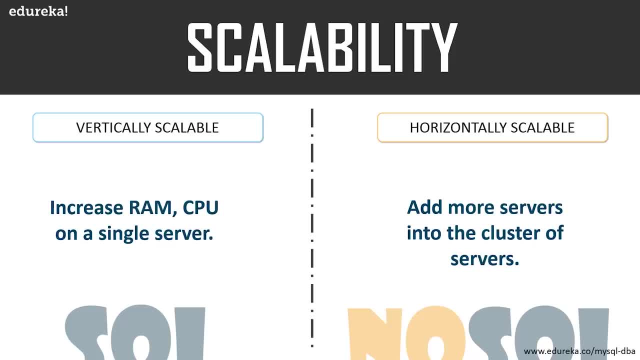 by optimizing your hardware requirements, such as increasing the CPU, RAM, SSD, etc. on a single server. on the other hand, the no sequel databases are horizontally scalable. You can do load balancing by adding more servers to your cluster so that, with the help of these servers, 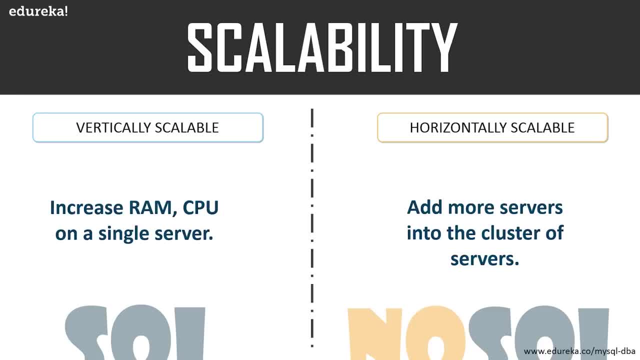 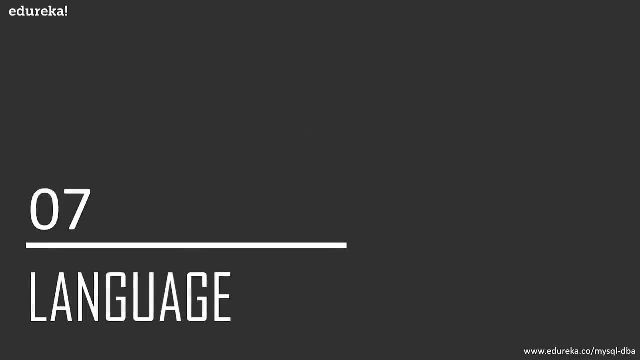 you can handle large traffic. So on the note of scalability, sequel is vertically scalable and no sequel is horizontally scalable. next We'll be comparing these databases based on language. The sequel databases have a specific language and it does not vary from database to database. 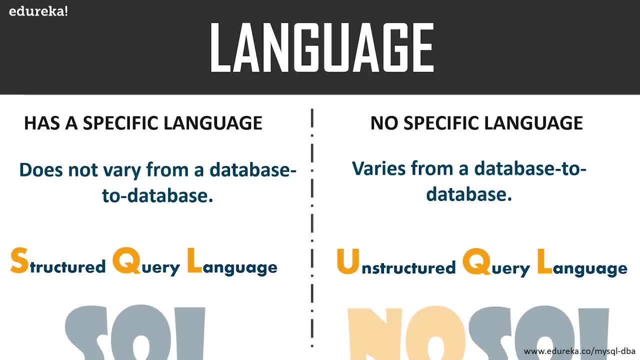 So basically, the sequel databases use the structured query language for defining and manipulating the data, which is very powerful. Coming to no sequel: the no sequel has no specific language and it varies from database to database. in the no sequel databases The queries are focused on the collection of documents. 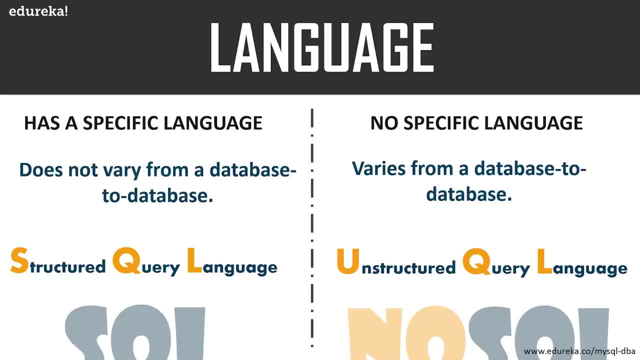 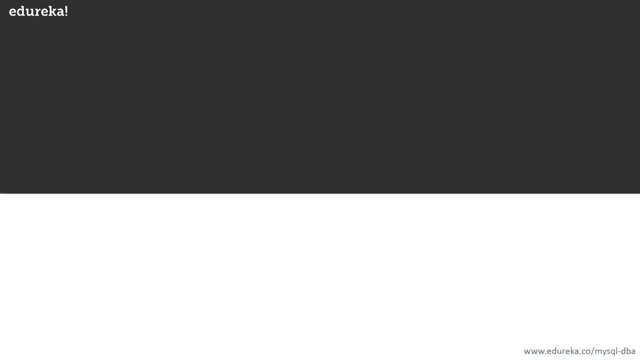 and sometimes the language used in no sequel is also called unstructured query language. So on the note of language guys, the sequel uses a proper, defined language, that is the structured query language, and no sequel has no specific language and the language differs from database to database. now moving 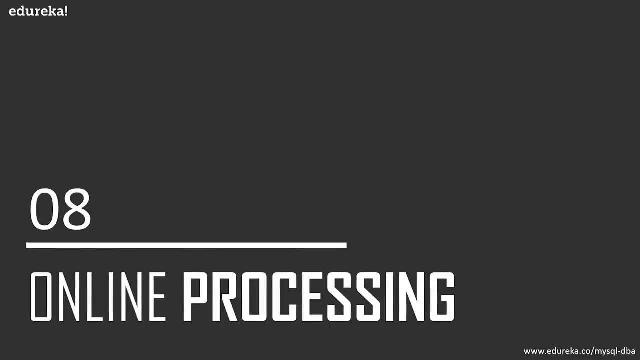 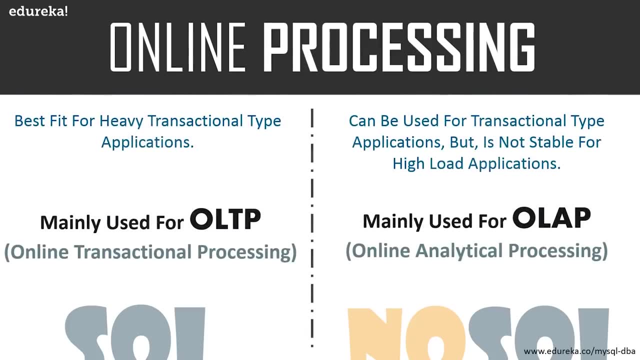 on to the next parameter, which is online processing. now, when we compare both these databases based on online processing, sequel databases are the best fit for heavy-duty transactional type applications as its most stable and promises the atomicity as well as the integrity of data, while you can definitely use no sequel. 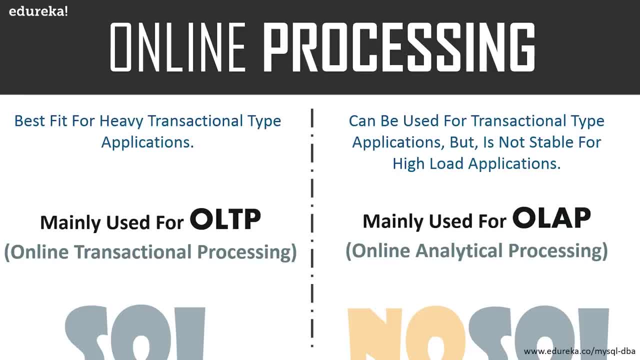 for transaction purpose, yet It is still not comparable and stable enough and high load for complex transactional applications. So you can understand by this that you know sequel is mainly used for OLTP, That is, basically online transactional processing, and no, sequel is mainly used for OLAP. 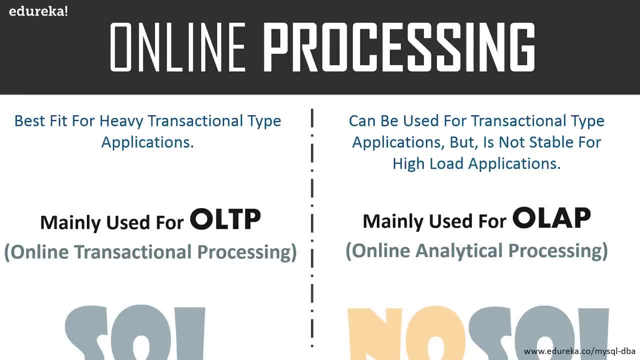 which is online analytical processing. So if I have to just explain these terms- OLTP and OLAP- for you, then OLTP is basically characterized by large number of short online transactions, such as insert, update and delete. the main emphasis for OLTP systems is to put on a very fast query processing. 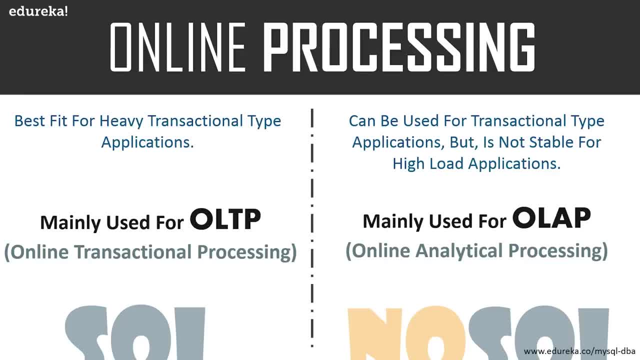 maintain data Integrity in multi-axis environments and an effectiveness measured by number of transactions per second. in OLTP databases There's proper, detailed and current data, and the schema used to store transactional database is, in the entity model, usually 3nf. now coming to OLAP. 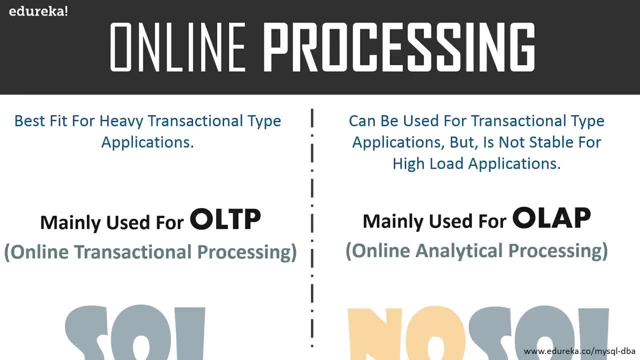 That is basically online analytical processing. This is basically characterized by relatively low volume of transactions, and queries are often very complex and involve aggregation. for OLAP systems, response time is an effectiveness measure and OLAP applications are widely used by data mining. So in the OLAP database there is aggregated historical data. 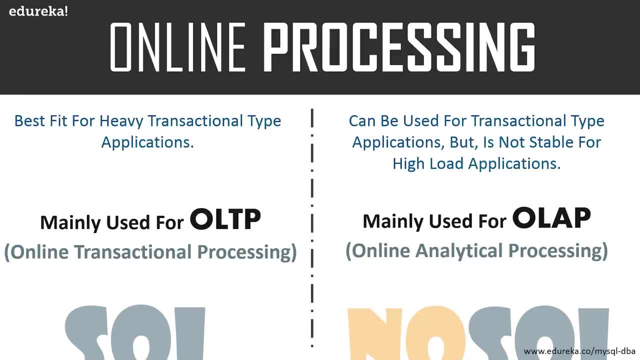 stored in multi-dimensional schemas, usually the star schema. So, guys, that was about OLTP and OLAP. So you can just understand this point that you know. sequel is mainly used for heavy transactional type applications and no. sequel is basically used for analytical processing and can definitely be used for transactional type applications. 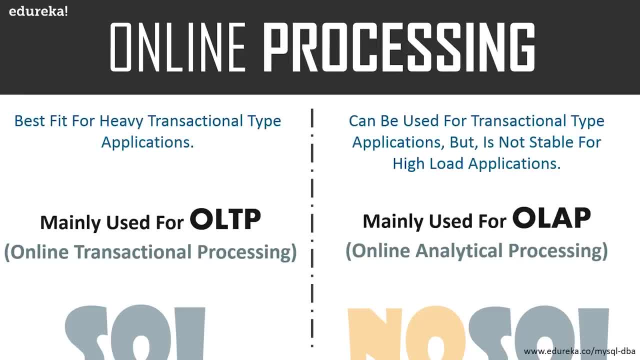 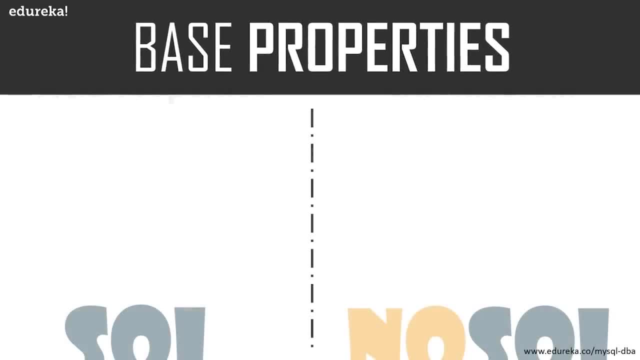 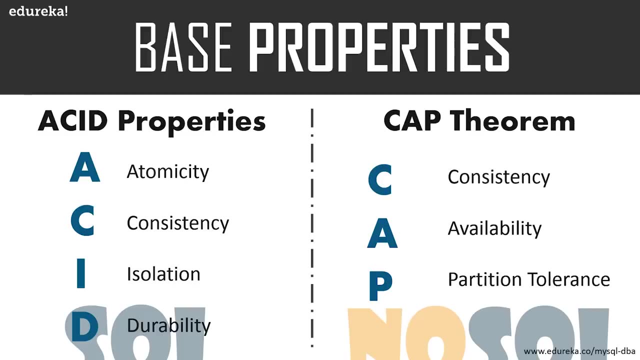 but yet it is still not stable for high load applications. So now the next point of comparison we have is base point: These properties- now sequel databases- emphasize on the asset properties, that is, the atomicity, consistency, isolation and durability, whereas the no sequel database follows the cap theorem, that is, the consistency availability. 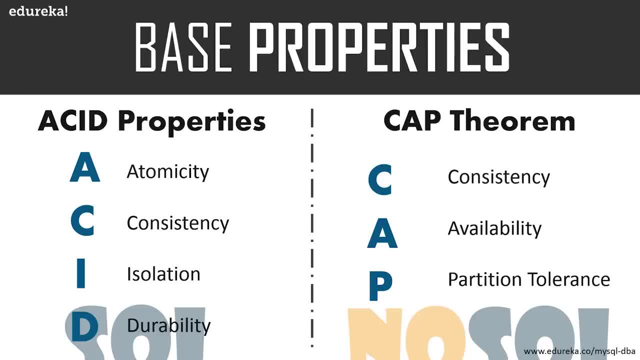 and partition tolerance. So let's talk about both of them one by one, starting with the asset properties. asset properties mainly stand for atomicity, consistency, isolation and durability. now, atomicity basically refers to the transactions that are completely done or failed, where the transaction refers to a single logical operation. 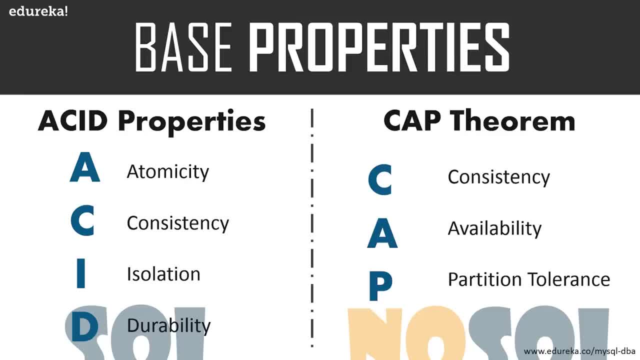 of data. now this basically means that you know, even if one part of the transaction phase, the entire transaction phase and the database state is left unchanged, coming to consistency. the consistency ensures that data must meet all the validation rules. in simple words, You can just say that you know your transaction never leaves. 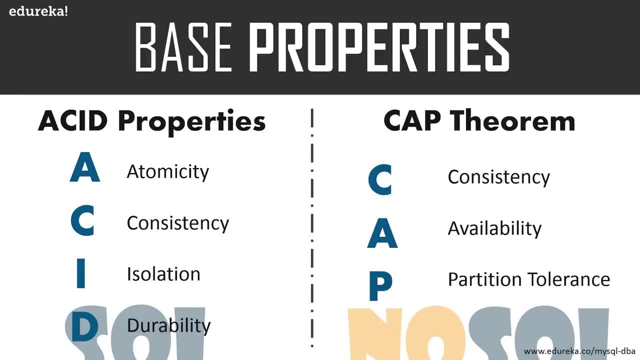 the database without completing its state, coming to isolation. The main goal for isolation is basically the concurrency control and finally, the durability. the durability means that you know if a transaction has been committed, it will occur whatever may come in between, such as the power loss, crash or any sort of error. 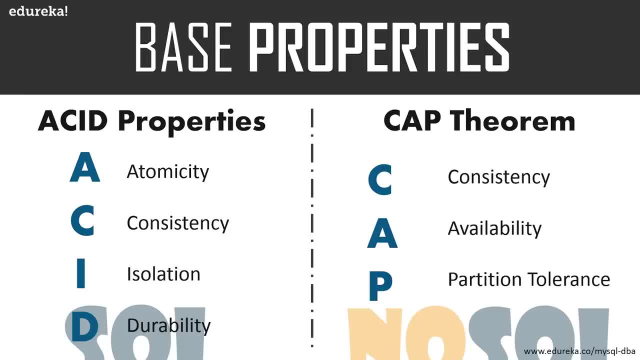 So, guys, that was about the asset properties. That is basically the atomicity, consistency, isolation and durability. coming to the cap theorem, the cap theorem, or the Eric Brewers theorem, states that you know, we can only achieve at most two out of three guarantees for a database. that is basically the consistency, availability. 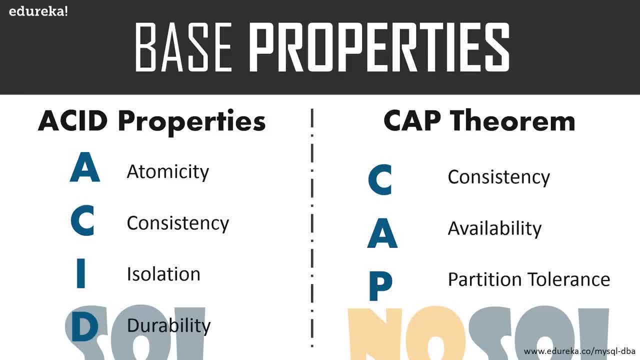 and partition tolerance. So here the consistency means that you know all the nodes in the network, See the same data at the same time, or the reader gets most recently written data coming to availability. availability is the guarantee that every request receives a response about whether it is successful or failed. 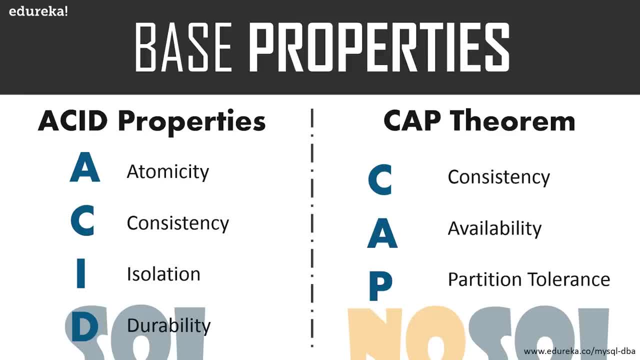 and the more number of users a system can cater to, a better is the availability coming to the partition tolerance. The partition tolerance is a guarantee that the system continues to operate despite arbitrary message loss or failure of any part of the system. in other words, even if there is a network outage in the data center. 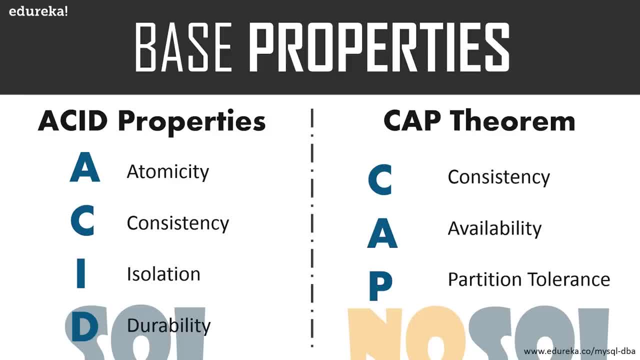 and some of the computers are unreachable till the system continues to perform. now, out of these three guarantees, that is, the consistency, availability and partition tolerance, No system can provide more than two guarantees. now, since in the case of distributed systems, the partition of Network is must, the trade-off is always. 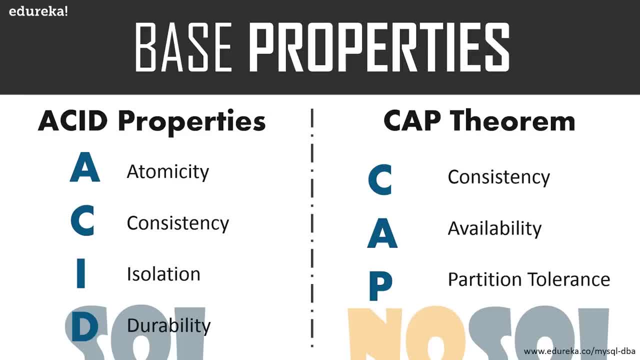 between consistency and availability. So you can just understand that. you know, no sequel cannot provide consistency and high availability to get. so, guys, that was about the base properties. sequel is completely based on the asset properties and no sequel is based on the cap theorem. Finally, the last, 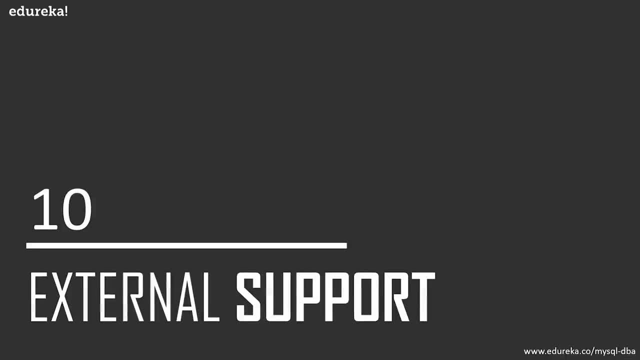 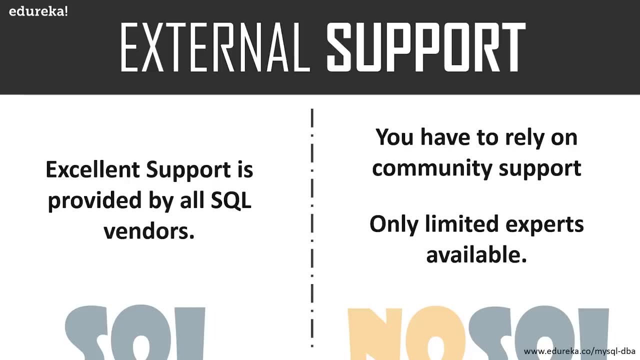 but not the least factor of comparison is external support. now external support is available for all sequel database from the vendors. There are also a lot of independent consultations who can help you with sequel database for a very large scale deployment. This is mainly due to since sequel has been 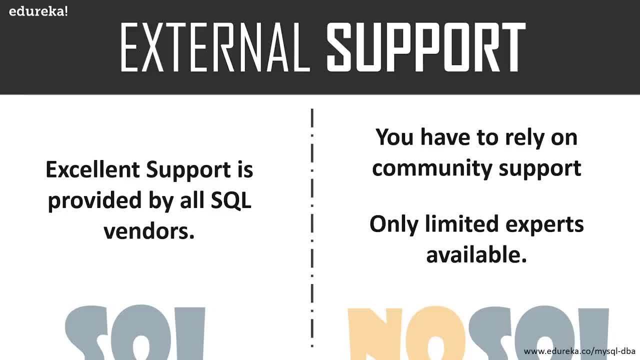 into existence in more than 40 years and people have been using sequel regularly, now coming to no sequel for some no sequel databases. You still have to rely on the community support and only limited outside experts are available for you to set up and deploy your large-scale. 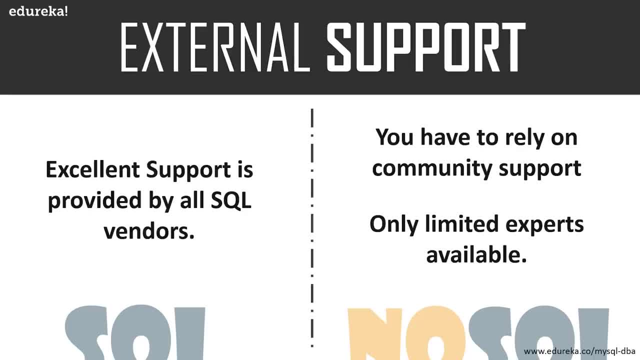 no sequel deployments. This is mainly because no sequel has come into existence and many of them haven't explored it yet. much So, folks. with this we come to an end of this phase of between sequel and no sequel. I hope all the comparison factors were clear to you guys now. 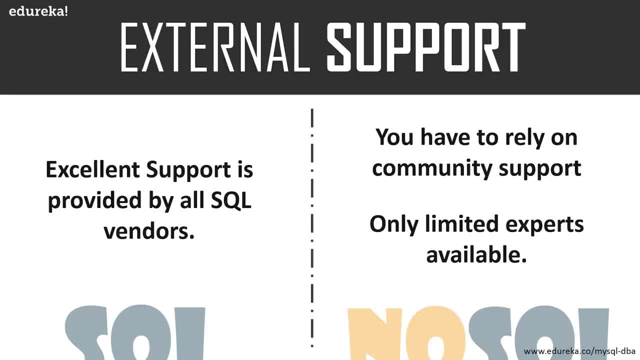 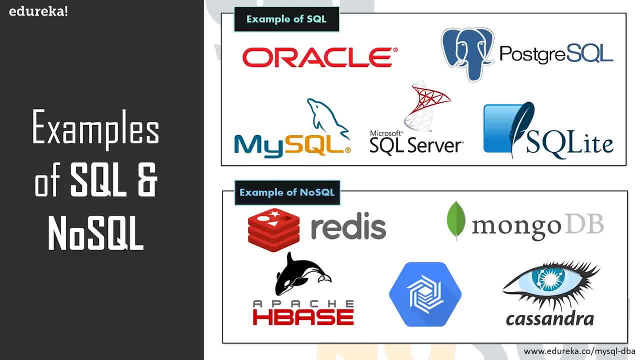 in this session. since we have discussed so much about sequel and no sequel, Let me just show you some examples of the same. So, as you can see on my screen, these are the examples for sequel and no sequel. So the popular examples for sequel are the Oracle, the Postgres, 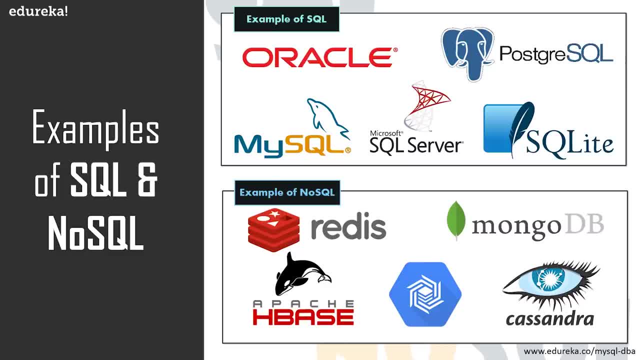 sequel, the my sequel, the Microsoft sequel server and sequel. right now, coming to the examples of no sequel. The examples of no sequel are Redis, MongoDB, Apache, HBase, big data table and Cassandra- now out of the lot. the most popular databases in today's market are basically the my sequel. 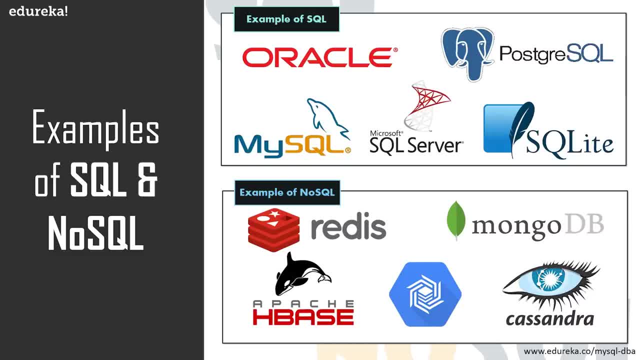 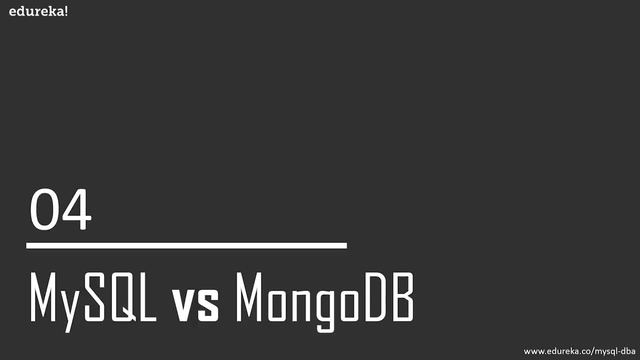 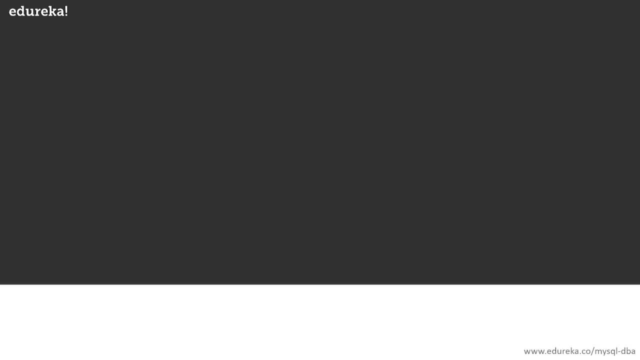 and MongoDB from the sequel and the no sequel sections. So next in this session will be comparing my sequel and MongoDB based on various parameters. Now, before I move on with the comparison of my sequel and MongoDB, let's first understand what is my sequel and what is MongoDB. starting with my sequel, 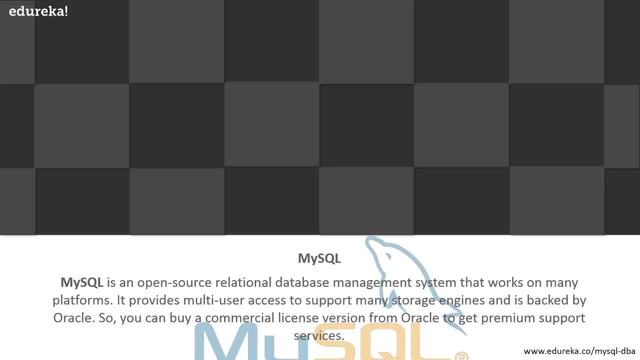 My sequel is an open-source relational database management system that works on many platforms. It provides multi-user access to support many storage engines and is backed by Oracle, So you can buy a commercial license version from Oracle to get premium support services. Now the features of my sequel, as you can see on my screen. 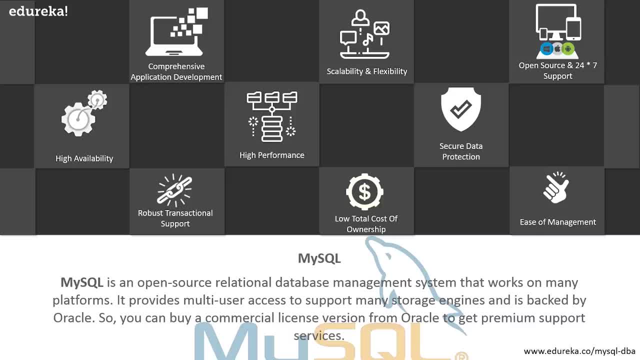 So basically, my sequel provides comprehensive application development, scalability and flexibility and it's open source and provides 24 into 7 support. provides high availability, high performance, support secures or data. provides robust transactional support, requires low total cost of ownership and provides ease of management in the coming to comprehensive application development. 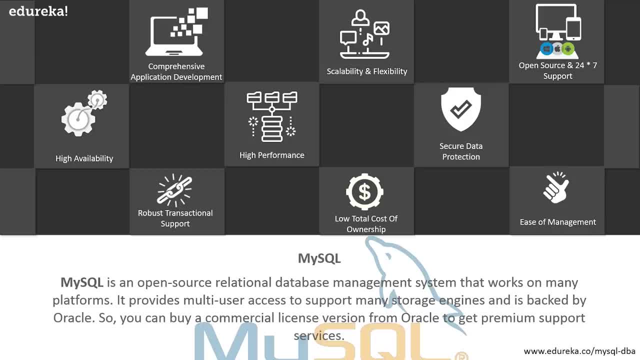 My sequel has plug-in libraries to embed the database into any application, So it basically supports stored procedures, triggers, functions, views and many more application development, coming to scalability and flexibility. with my sequel, You can run deeply embedded applications and create data warehouses holding a humongous amount. 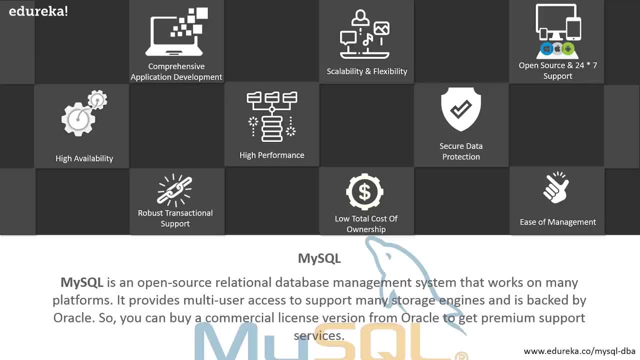 of data. next, talking about open source and 24 into 7 support, this relation database management system can be used on any platform and offers 24 into 7 support for open source and Enterprise Edition. talking about high availability, my sequel can run high-speed master slave. 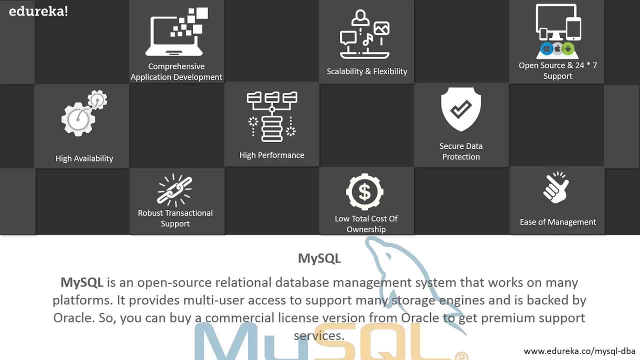 replication configurations and it offers various cluster servers. talking about high performance, my sequel provides fast load utilities with distinct memory caches and tables index partitioning. next, about data protection: my sequel supports powerful mechanisms to ensure that only authorized users have access to the databases. next, talking about robust transactional support: 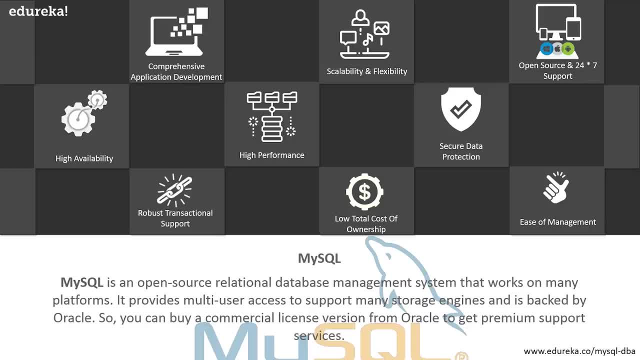 My sequel holds the asset properties, that is, basically the atomicity, consistency, isolation and durability properties, and allows distributed multi-version support. and talking about low total cost of ownership, My sequel make sure that you need reduces the licensing costs and Hardware expenditures. and talking about, finally, the ease of management. this software can be easily downloaded. 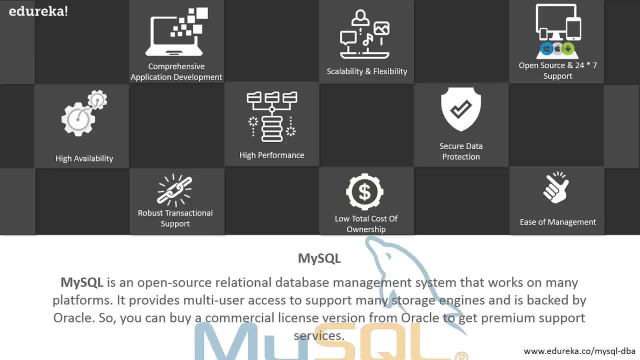 and also uses an event scheduler to schedule a task automatically. So, guys, the features of my sequel are basically the comprehensive application development, The scalability and flexibility, open source and 24-7 support, high availability, high performance, secure data protection, robust transactional support, low total cost of ownership. 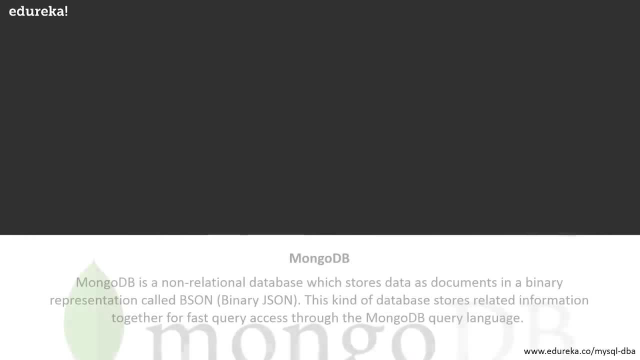 and ease of management. now coming to MongoDB. MongoDB is a non-relational database with stores data as documents in a binary representation called BSON, that is basically binary JSON. this kind of database stores related information together for fast query access to the MongoDB query language. The features of MongoDB are as you can see on my screen. 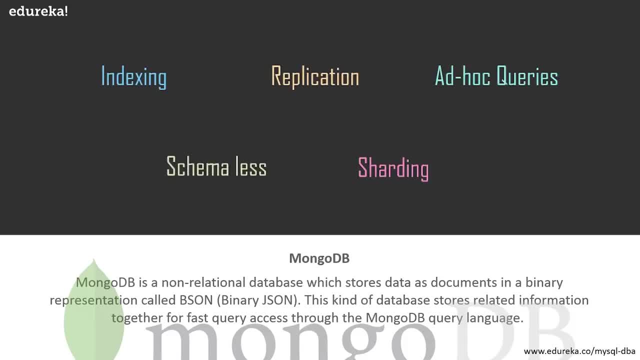 that is, indexing, replication, ad-hoc query schema list and sharding. talking about indexing, MongoDB: indexes are created in order to improve the search performance. next, talking about replication, MongoDB distributes the data across different machines. coming to ad-hoc queries, MongoDB supports ad-hoc queries by indexing the BSON documents. 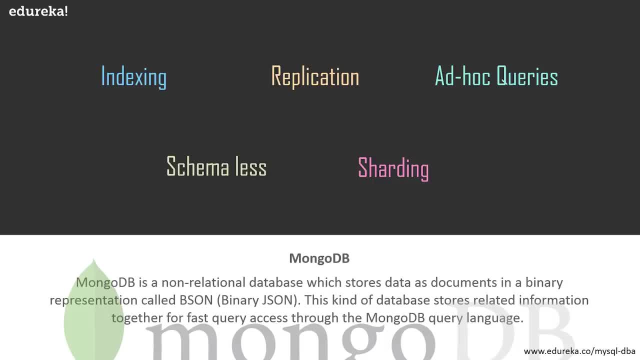 and uses a unique query language. coming to schema list, It's very flexible because it's schema list database and is written in C++. and talking about sharding, MongoDB uses sharding to enable deployments with large data sets and high throughput operations. So, guys, these are the mainly five features of MongoDB. 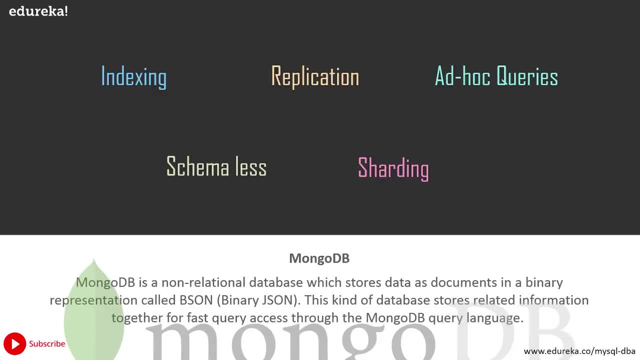 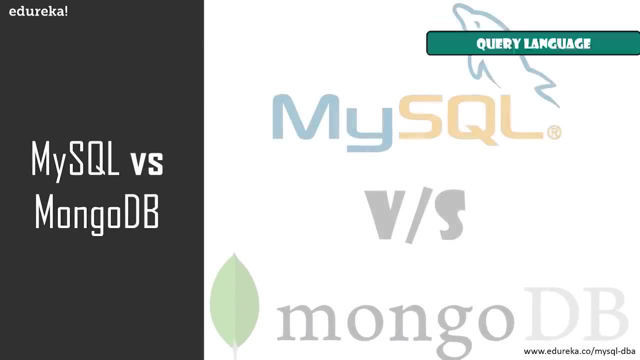 that is, indexing, replication, ad-hoc query schema list and sharding. so there's now that you know what my sequel is and what MongoDB is. let's compare these two databases based on the grounds that you can see on the screen. that is, the query language to flexibility of schema, the relationships, security, performance. 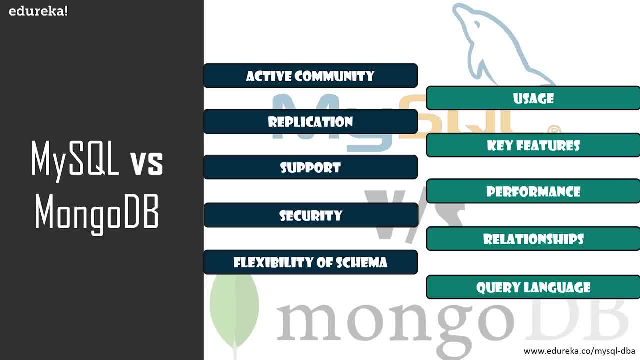 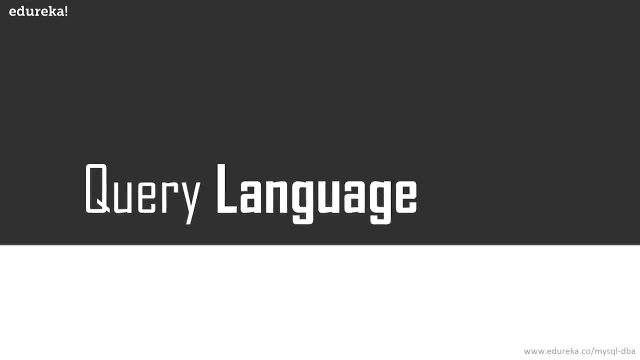 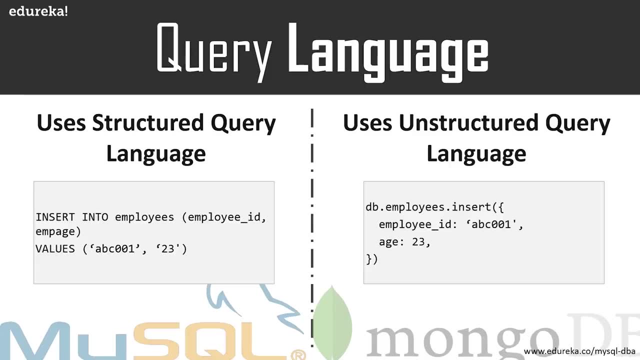 support, Key features, replication, usage and active community. So now let's get into detail with the first comparison factor, that is, the query language. now my sequel uses the structured query language to communicate with the database. Not only is it simple, It is also very powerful language, which consists: 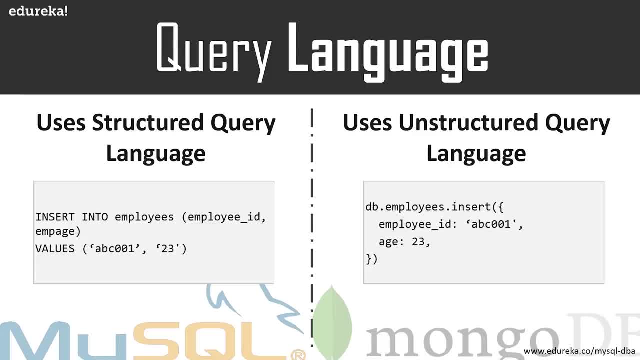 of mainly two parts, that is, the data definition language and the data manipulation language. MongoDB, on the other hand, uses an unstructured query language. to build a query in Jason documents, You need to specify a document with various properties You wish the results to match. it is typically executed. 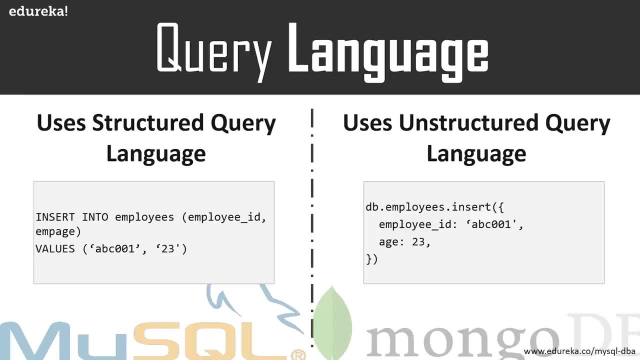 using a very rich set of operators that are linked with each other. using Jason, now, MongoTV treats each property as having an implicit boolean and it basically also supports boolean or queries. but you must definitely use the special operator dollar or to achieve it. So to make you understand better. 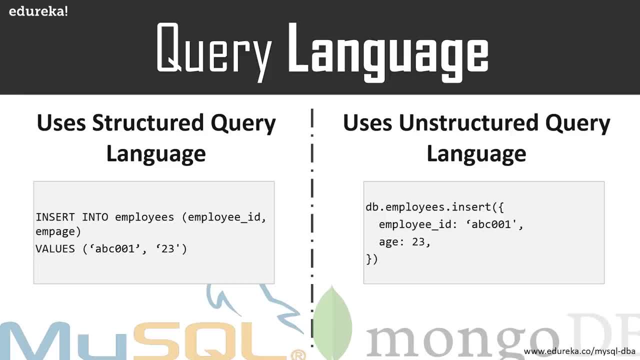 I've considered the example on the screen. So to insert the data into the employees table in the sequel query you just have to type an insert into employees that is basically your table name and insert into is your sequel syntax. and then you mentioned the column names. 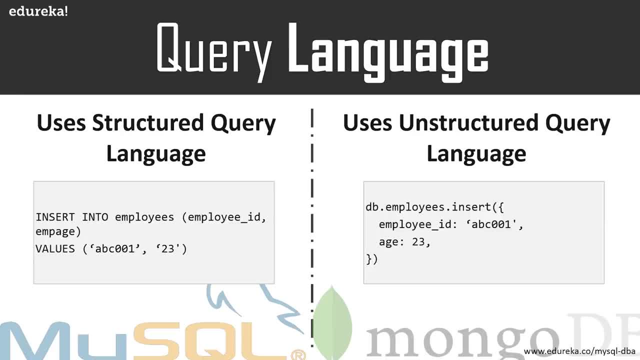 that is, the employee ID and employee age, and then you use the sequel syntax, that is, the values, and mention the values for the fields. So to just insert data into the table you mentioned, insert into employees employee ID, employee age values, and then you mentioned the values now. similarly, 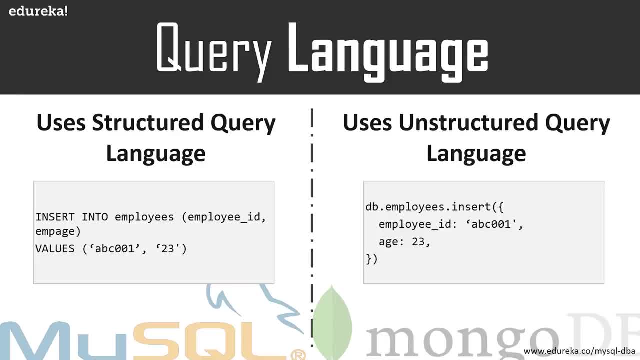 in the same scenario. If you wish to insert the data into a collection which is stored in the MongoDB database, What you simply have to do is you have to mention DB dot employees or insert where employees is the collection name, and then you have to mention employee ID. 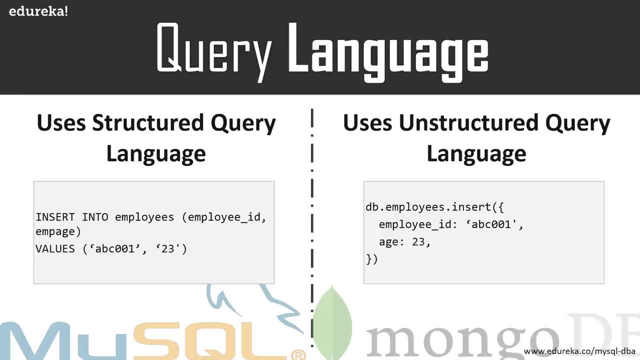 and then mention the value, and then mention again age and the value. So, basically over here, employee ID and age are basically the fields. So, guys, this is how you know the query language between my sequel and MongoDB differs. next We'll be comparing these databases based. 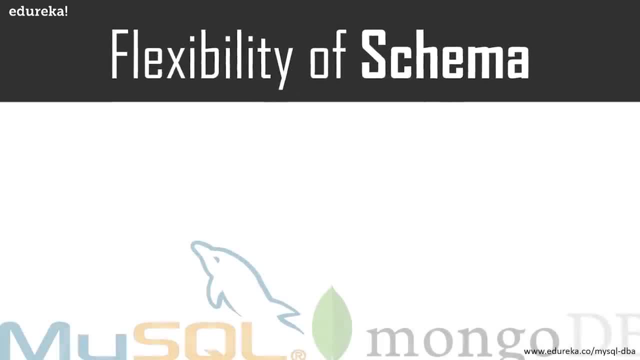 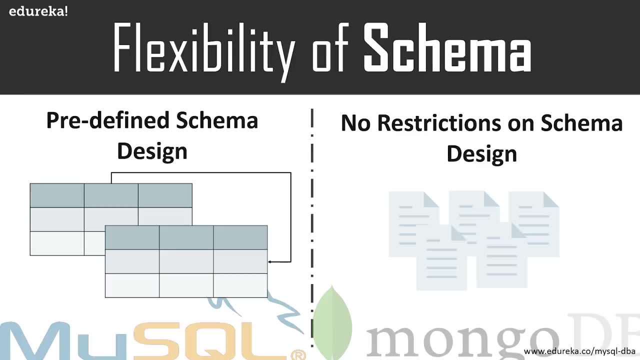 on the flexibility of schema. now, in the perspective of flexibility of schema, Let me tell you that you know, before you can store anything in my sequel, you need to clearly to find tables and columns, and every row in the table should have the same column. Now, this is basically. 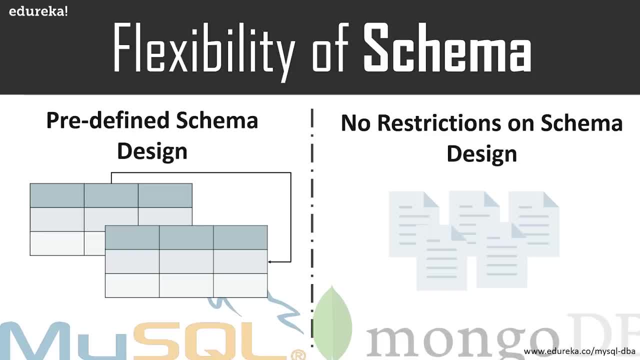 because there isn't much space for flexibility in the manner of storing data If you follow normalization. for example, if you have an employee database, you need to create a table which can hold the date of employees. Now this table can have many attribute values. 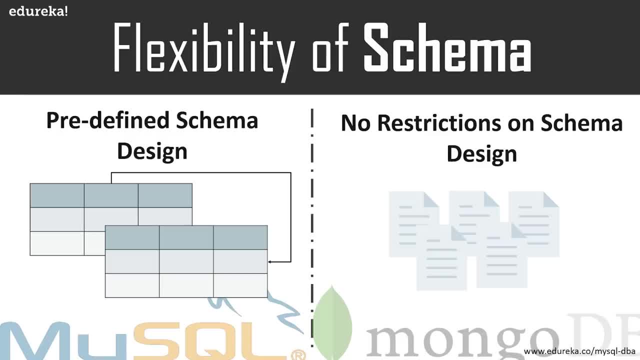 such as the employee ID, employee name and so on. now, Similarly, talking about MongoDB, one of the best things about MongoDB is that you know there are no restrictions on the schema design, so you can directly drop a couple of documents within a collection and it isn't necessary to have any relations. 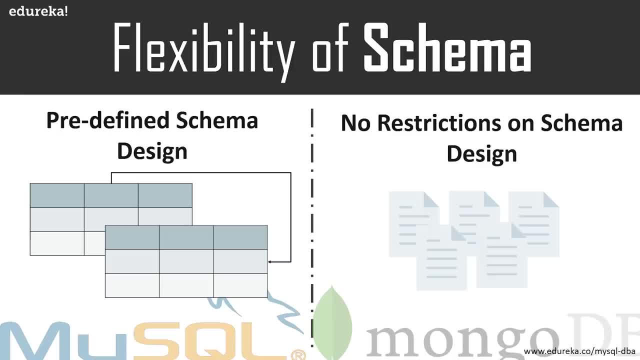 between those documents. Now, the only restriction with MongoDB is that you need to frequently optimize your schema based on how the application will be accessing the data. now MongoDB stores the data in the JSON type manner. So, if you consider the previous example, there is the employee table. the data in MongoDB would be stored. 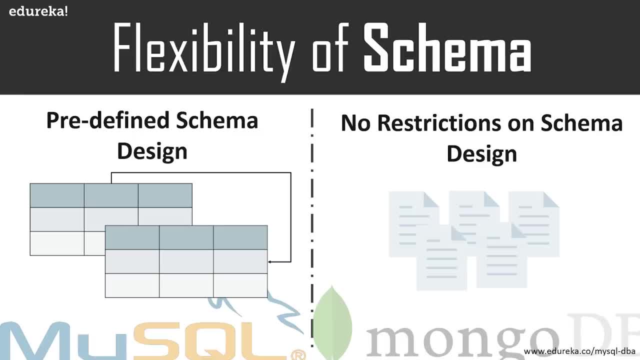 as you know, employee ID- and then we have to mention the employee ID. that is basically the value for employee ID, then employee name, and then you have to mention the employee name, employee age and so on. So basically this will be considered as a document, and now these documents can be stored in a collection as well. 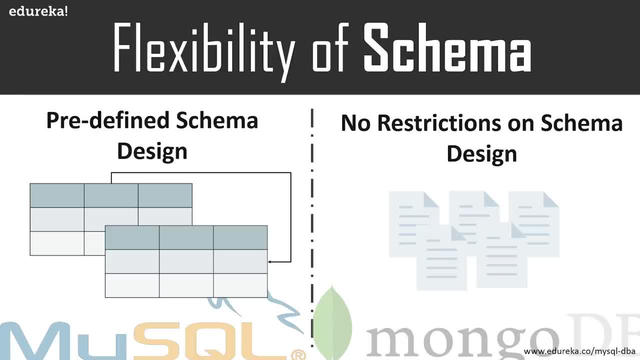 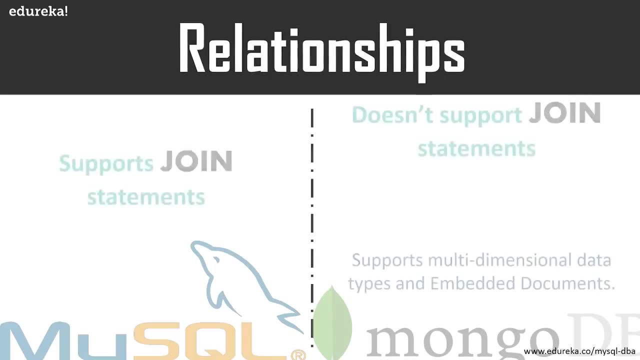 So, basically, MongoDB creates schema list documents which can store any information you want, though It may cause problems with the data consistency, whereas the my sequel follows a strict schema template. now moving on to the next parameter, which is relationships. now, when we talk about relationships, my sequel supports the join operations. 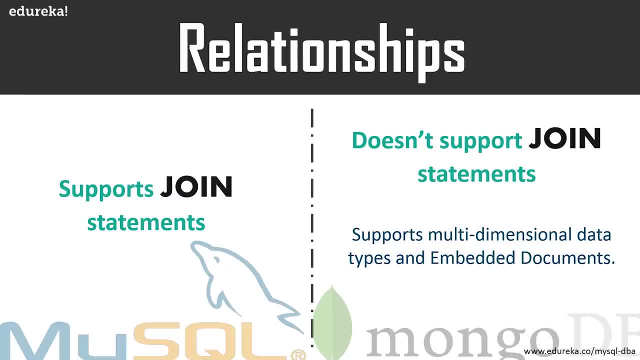 So, to explain you in simple terms, join makes the relational database relational. So basically, the join allows the user to link the data from two or more tables in a single query with the help of the select command. So, for example, if you want to retrieve the data from the employee, 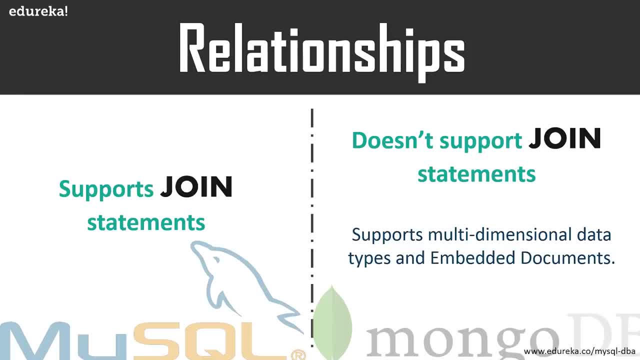 in the projects table, based on the matching column. you can easily obtain the desired data by applying any type of joints, just the inner left, right or full, based on your need. now coming to MongoDB. Well, MongoDB does not support the joint statements, but it supports the multi-dimensional data types. 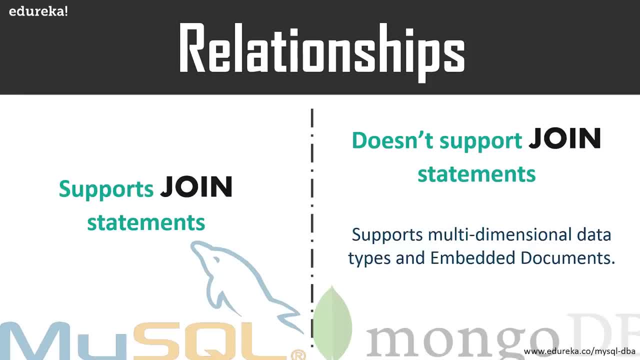 such as areas and even other documents. So the placement of one document inside another document is basically known as the embedding of document, and MongoDB supports the embedding of documents. So, talking about relationships, guys, my sequel supports the joint statements and the MongoDB does not support any joint statements. next, 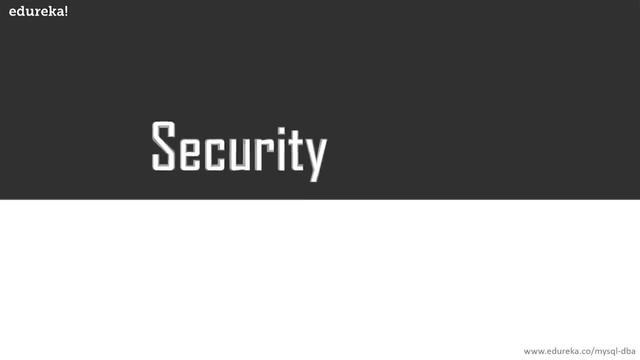 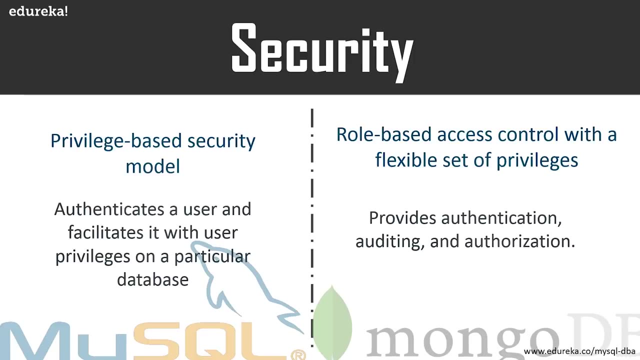 Let's discuss the security factor for both of them. Now, talking about my sequel first. my sequel uses a privilege based security model. This means that you know it basically authenticates a user and facilitates it with the user privileges on a particular database, such as create, select, insert, update. 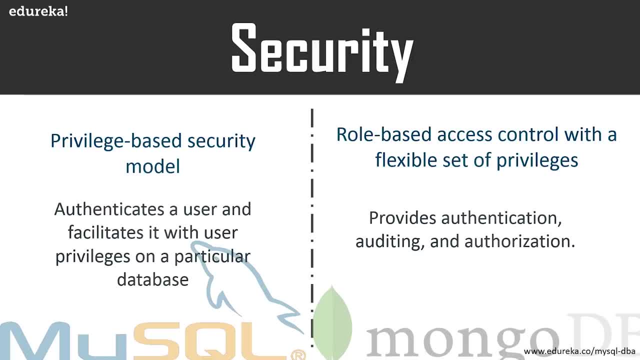 and so on. now coming to MongoDB. MongoDB uses a role-based access control with the flexible set of privileges. its security features basically include the authentication, auditing and authorization. not only this, but it is also possible to use the transport layer, security and the secure socket layer for encryption purposes in MongoDB. 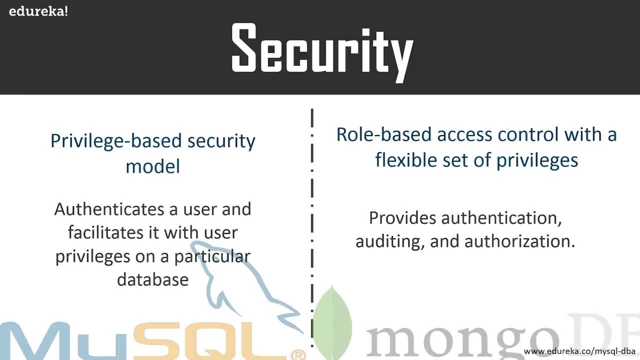 So, basically, this ensures that unit is only accessible and read it by an intended client. No other client can go through the documents. So, guys, that's how the security is provided in my sequel and MongoDB. Now let's move forward to the next factor of comparison. 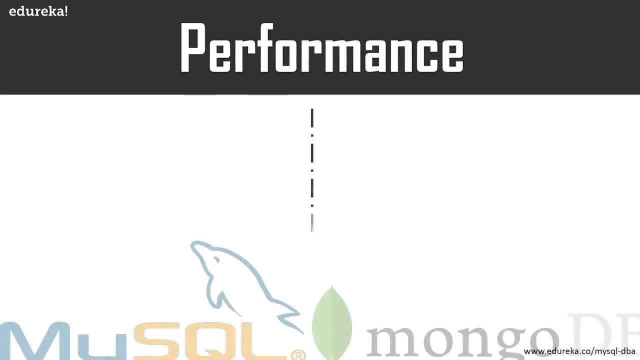 that is performance. So I'm comparing my sequel and MongoDB on this parameter. My sequel is quite slower in comparison to MongoDB when it comes to dealing with the large databases. This is mainly because, you know my sequel can't cope up with large and unstructured amounts of data. 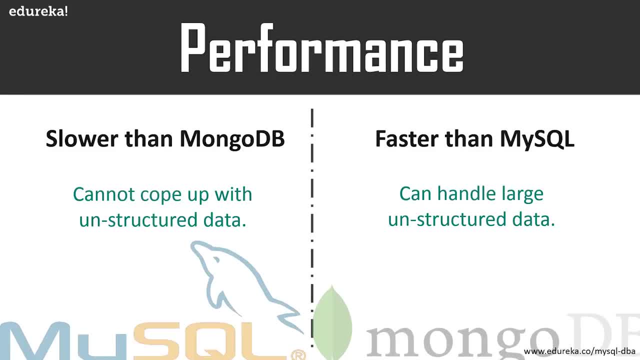 Whereas MongoDB can. so that's the reason, guys, MongoDB is much faster than my sequel. now, talking about MongoDB, MongoDB has the ability to handle large unstructured data. It's much faster than my sequel because it allows the users to query in a different manner that is more sensitive to workload. 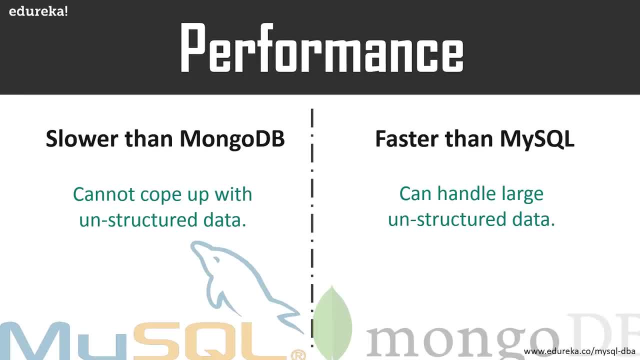 But, yes, there is as such no Benchmark on. you know which database is faster, because you know only your demands. your data and your infrastructure can tell what you need and which database can provide you the output faster. So, guys, that was about performance. next, We'll be comparing these databases based on support. Well, both of them offer excellent support 24: 7 for security fixes, maintenance releases, bug fixes, patches and updates. So there is, as such, no difference between both of them based on this parameter, as both of them offer good support. 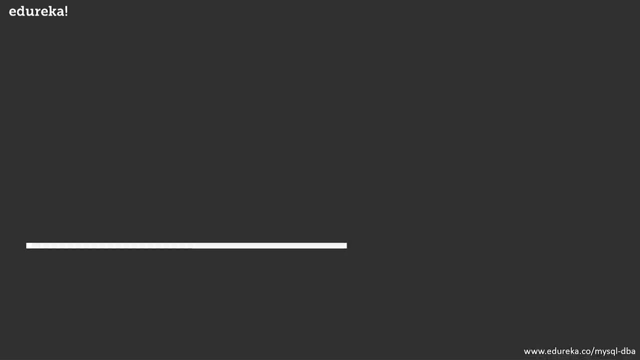 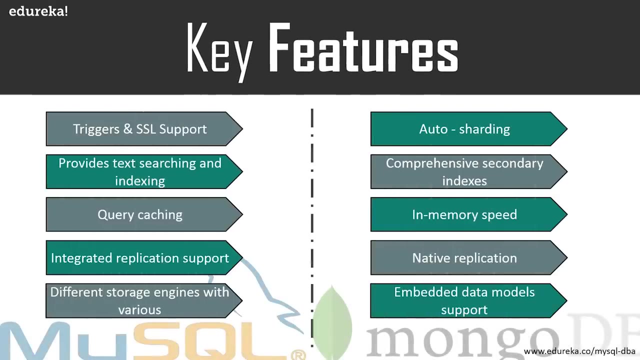 So, guys, that was about support. now moving on to the next parameter, which is key features. the key features of my sequel in MongoDB are, as you can see on my screen. Let's start with my sequel first. the key features of my sequel are mainly triggers. 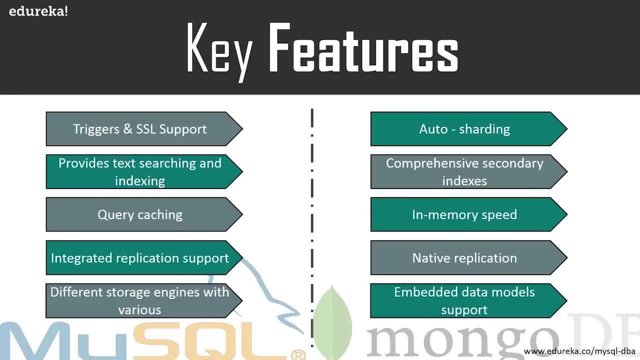 and SSS support, provides text searching and indexing, also allows query caching, provides integrated replication support and also provides different storage engines. So, guys, these were the key features of my sequel, not talking about MongoDB. MongoDB supports auto sharding, comprehensive secondary indexes in memory speed, native replication. 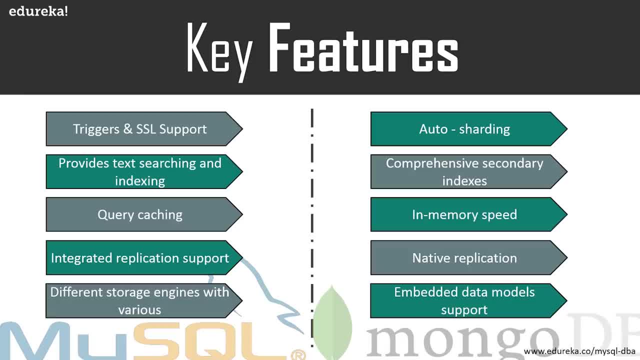 and embedded data model support. So these were a few features of my sequel and MongoDB. So, yes, there are various differences between both these databases, but there are few key features, you know, which help both my sequel and MongoDB to win in their own market. now 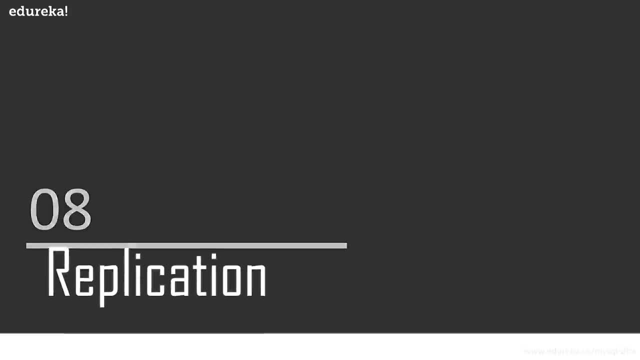 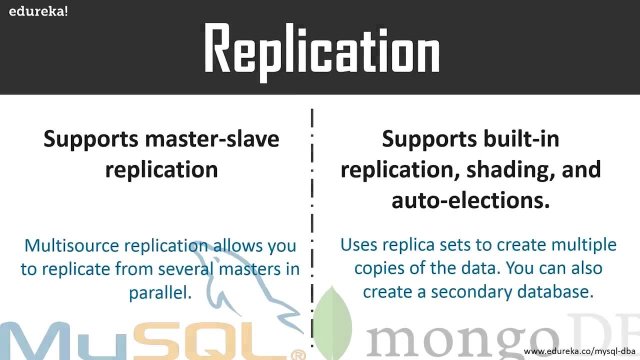 Next point of comparison we have is replication. now my sequel supports the master slave replication and the master master application as of my sequel, 5.7.6 and later, and this kind of multi-source replication allows you to replicate from several Masters. and paler talking about MongoDB, MongoDB supports the built-in. 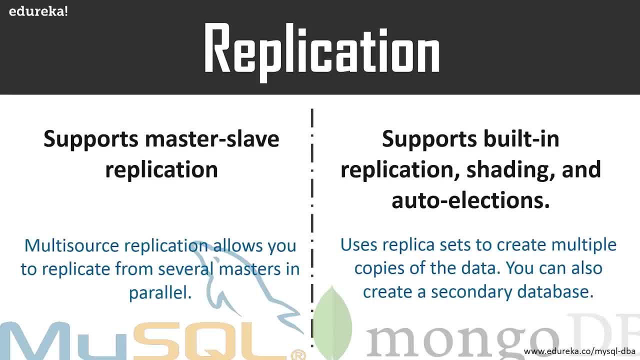 replication, sharding and Auto elections. So by using Auto elections, you can set up a secondary database to automatically take over if the primary database fails. so sharding allows for horizontal scaling, which is difficult to implement in my sequel, as my sequel is vertically scalable. not only this, 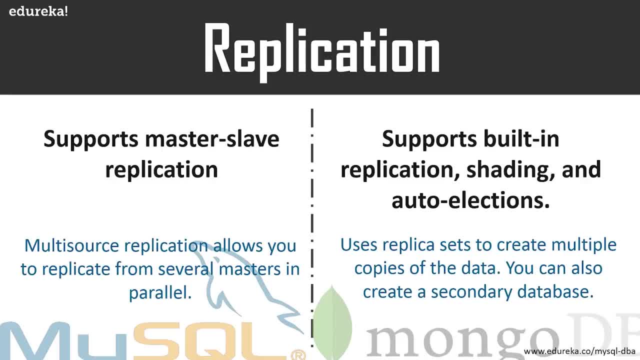 but MongoDB also uses replica sets to create multiple copies of data, So each member of the replica set can have the role of primary or secondary at any point in the process, and the read and writes are done on the primary replica by default and then replicated to the secondary replicas. 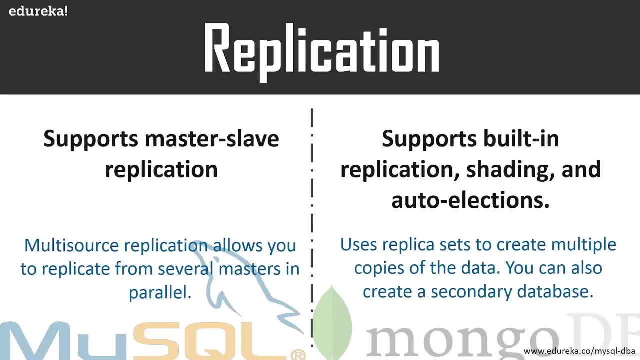 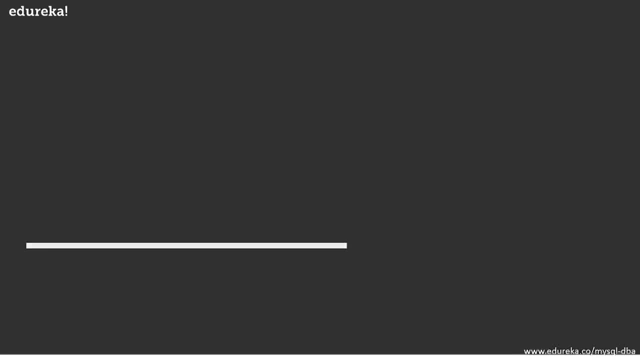 So, guys, this was about the replication. my sequel supports the master slave replication and the MongoDB supports built-in replication, sharding and Auto elections. next will be comparing these tools based on usage. now for this factor, I'm going to tell you where you can use my sequel and MongoDB. 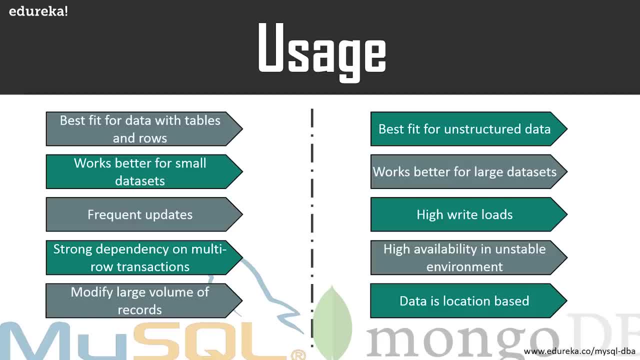 So let's start with my sequel first. my sequel is the best fit for data with tables and rows. This works better for small data sets and allows frequent updates. my sequel is also used for strong dependency on multi-door transactions and is also used when you want to modify large volumes. 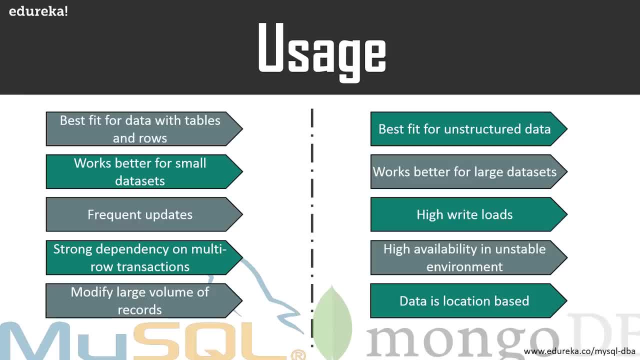 of records. talking about MongoDB, MongoDB best fits for unstructured data And, what's better, for large data sets. This is also used when you have high right loads and high availability in unstable environment and the data is completely location based. So this was about my sequel and MongoDB guys. my sequel mainly. 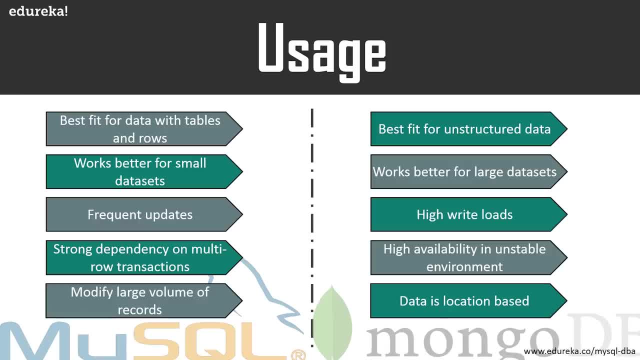 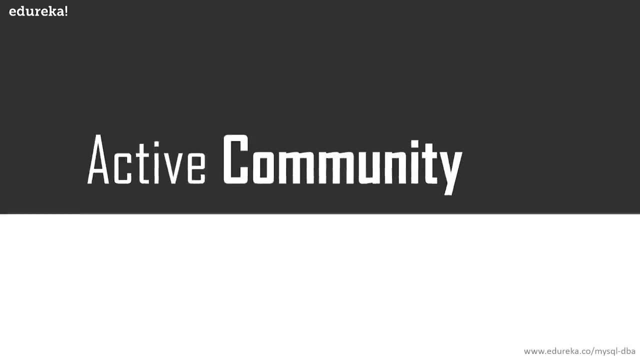 best fits for data with tables and rows, and MongoDB best fits for unstructured data. Finally, the last but not the least factor of comparison is the active community. the my sequel database is mainly owned and maintained by the Oracle Corporation, So they offer a developer zone. 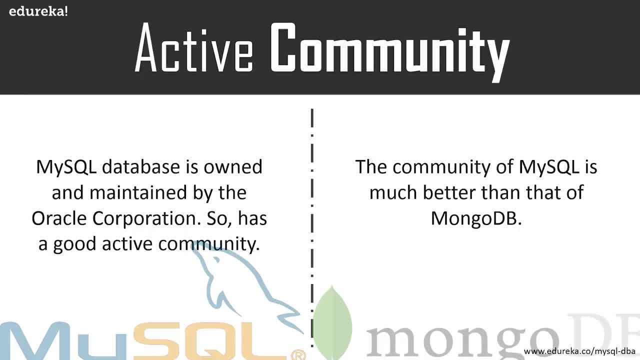 on the my sequel Website and the community for my sequel is, I would say, much better than that of MongoDB. So if you want to support both of them, offer good support. but yes, if you talk about active community, then my sequel has a better active community. 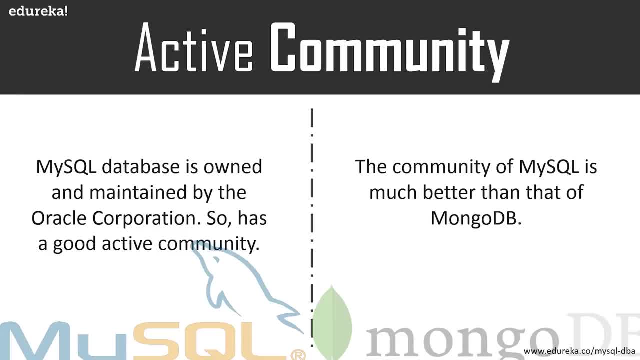 than compared to MongoDB. So, guys, now that I've told you so much about my sequel and MongoDB, let me just shift to my, my sequel workbench and MongoDB compass, so that I show you how you can create tables and databases in my sequel and how you can create databases and collections in MongoDB. 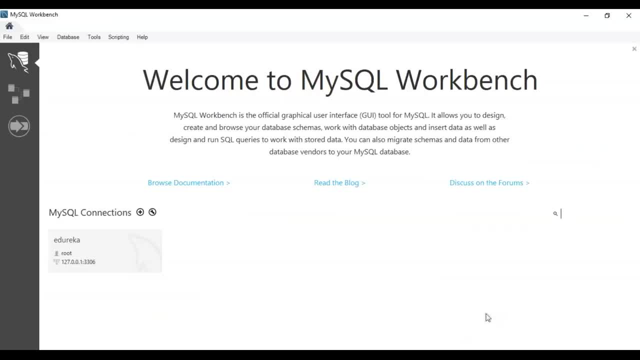 So first we'll be looking into my sequel. So for that, I'll open my my sequel workbench. So, as you can see on my screen, this is my my sequel workbench. So I'm just going to open my connection. So, guys, this is how your my sequel workbench looks now. 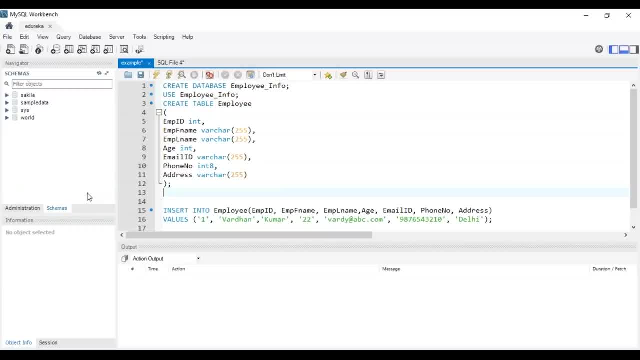 to show you how you can use my sequel. I've already written the command, So I'm just going to tell you how you can use them. So to create a database, I've used to query, create database and I've mentioned the database name, that is, employee info. 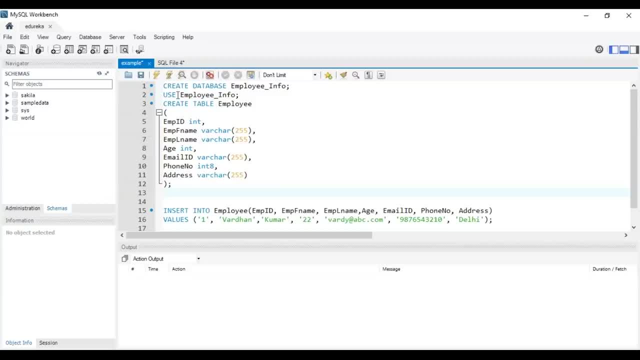 So this is a sequel language, guys, where you know create and database are the sequel syntax and employee info is the data parameter. So I'm going to just execute this particular query now. once the query is executed, you can clearly see that you know the database has been created now. 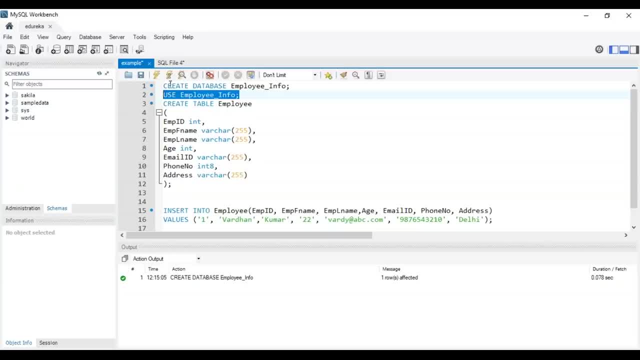 to use this database. You can just directly use database name, that is, employee info. So if I just execute this query again, you'll clearly see that you know we'll be using this particular database now to create a table inside this particular database. 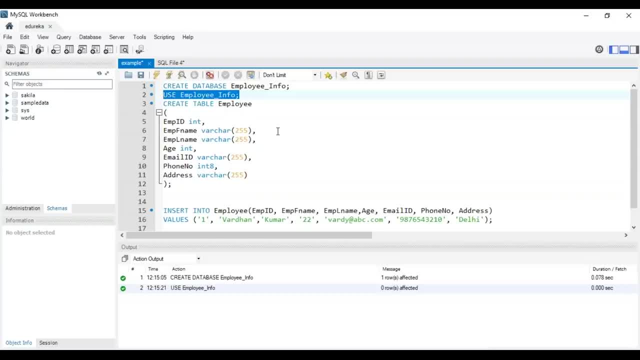 You can use the query like you know, create table, table name and then you mentioned all the field names and the data types. right, So we are. I have different field names, like the employee ID: Employee first name, last name, age, email ID, phone number. 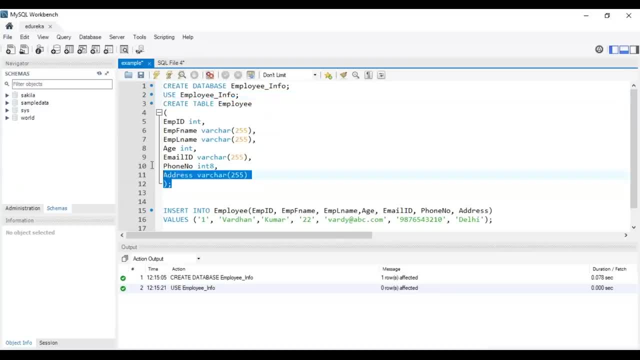 and address and their specific data types, right? So I'm going to just execute this particular query. So once I execute this particular query, you can see that you know a table has been created. So now, if we just look into our databases, 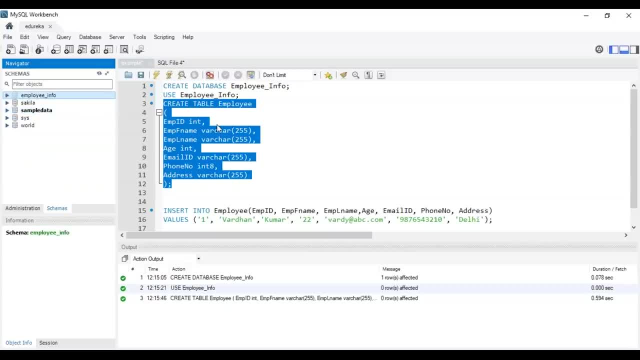 we have a database that is employee info and then we have a table inside it. now to insert data into the table, What you can use is you can just use the query insert into table name that is employee over here. mention all the field names, then use the sequel syntax keyword values. 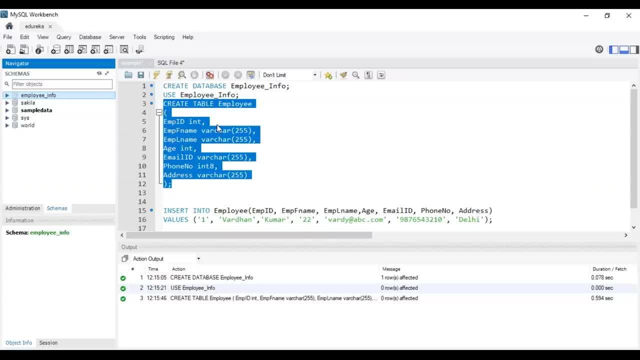 and then mention all the values right. So we have written a query as insert into employee: employee ID: first name, last name, age, email ID, phone number, address values, and then I've mentioned the values right. So I'm going to just execute this particular query. 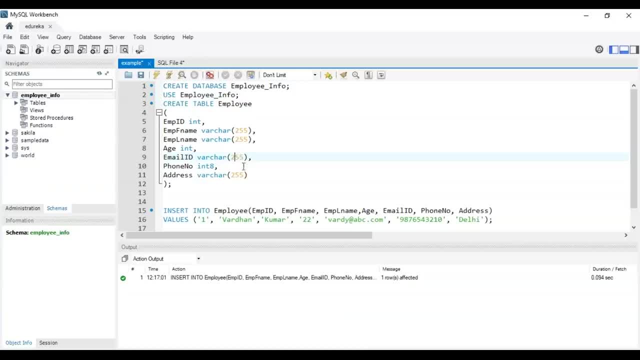 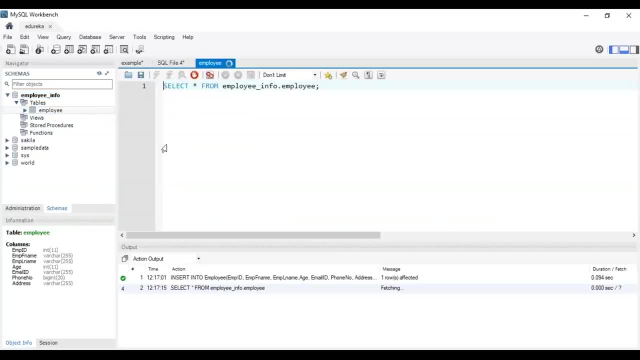 So once the query has been executed, you can clearly see that you know data has been inserted into the table. So I'll just go to the employee info table, go to the tables option, go to employee and then I'm going to just look into the table. 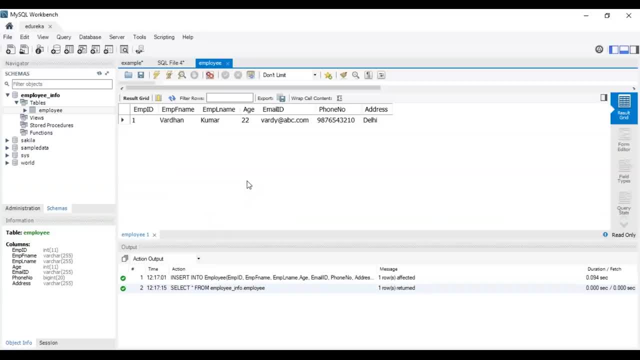 So when I just check into the option of view, you can clearly see that you know our first record has been inserted. So, guys, that's how it's really simple to use my sequel and, with the help of my sequel workbench, you get the GUI experience. 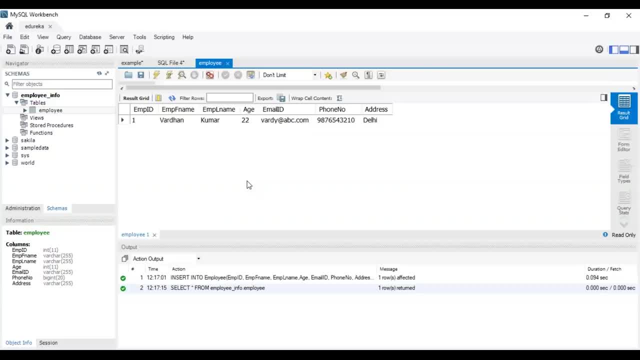 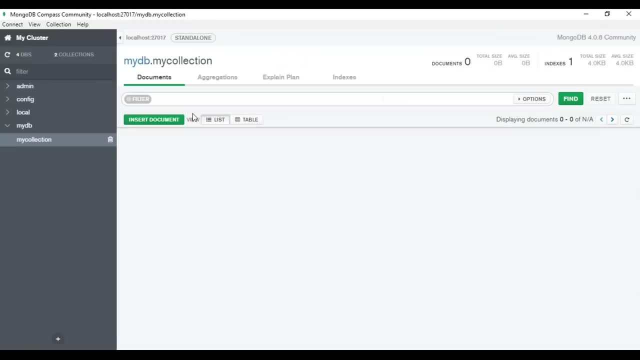 you know where you can easily mention your required queries and then get the outputs right. so that was about my sequel workbench guys now shifting to MongoDB compass. So, guys, this is how the MongoDB compass looks. So, basically, I've already created a database. now 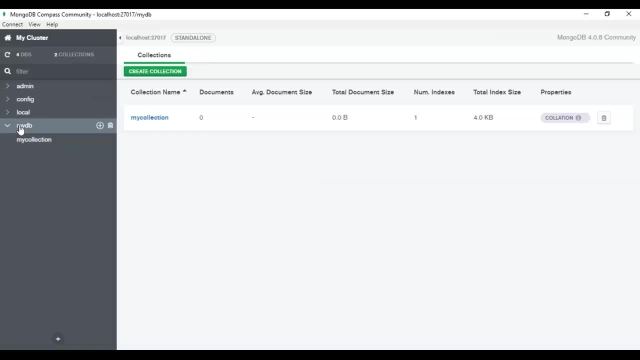 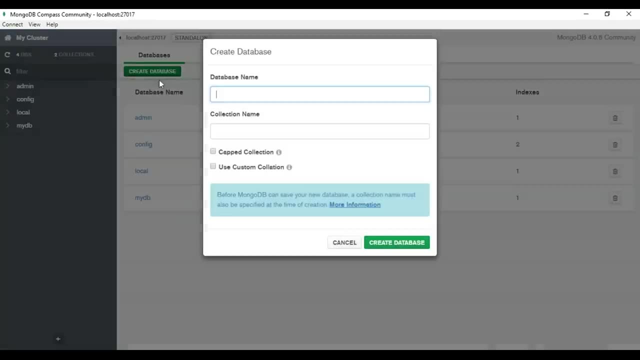 if you just wish to go and check how a database has been created, what you can simply do is you can go over here to my cluster and once you go to my cluster, you get an option of create database. right, So I'm just going to create a database. 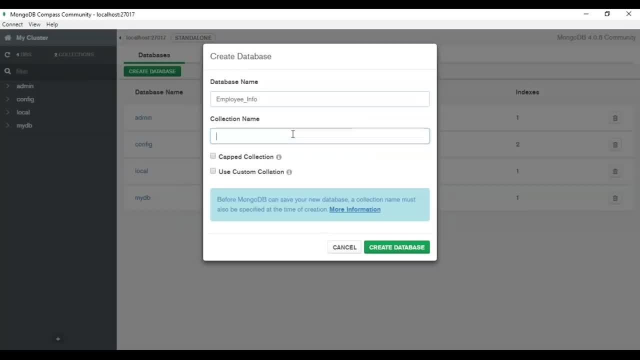 So let's say I mention it to be employee info and then over here, since I've told you, database has collections and then a collections have documents. So basically, a group of documents is collections and a group of collections is a database. I'm going to mention my first collection name. 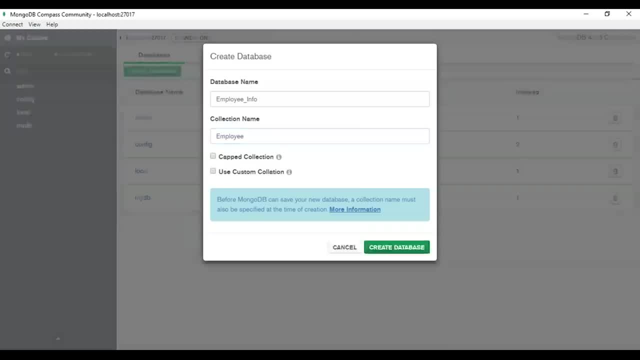 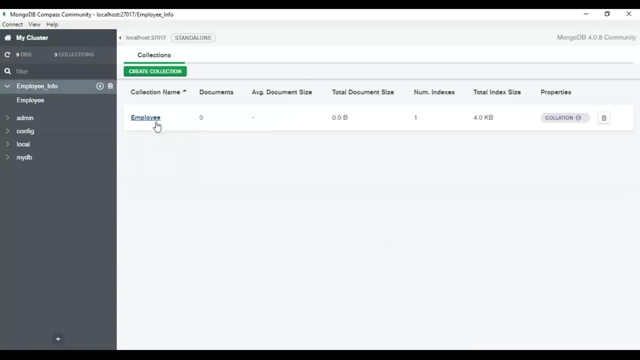 Let's say you know employee and then I'm going to just click on create database. So once I click on create database, you can clearly see that you know my database has been created. that is employee info. So I'll click on this. 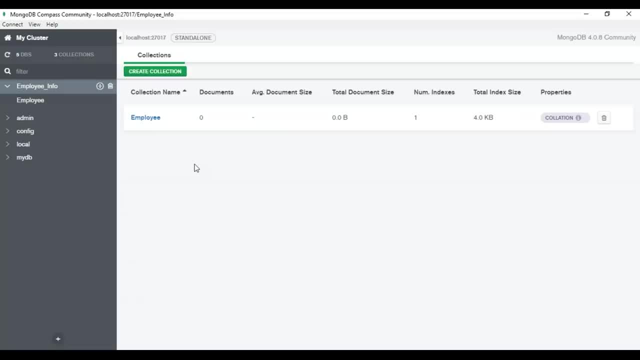 and you'll see that. you know I already have a predefined collection created. Now, apart from this, you can also have a number of collections to be created, But since I'm just showing you how you can use Mongo TV, I'm not going to create many more collections. 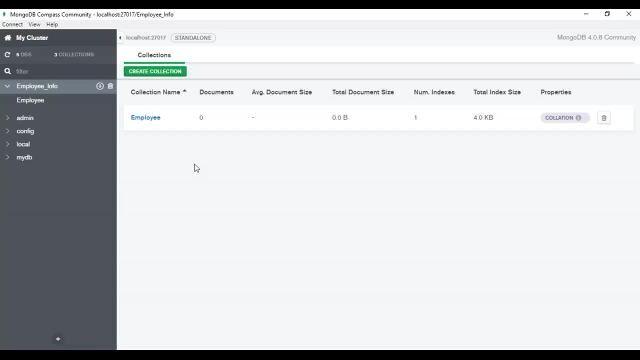 This is just a single collection that I've already created. Now what you can do is you can again create documents inside this particular collection. to do that, You have to click on this collection- that is the employee collection, and over here you get an option for insert document right. 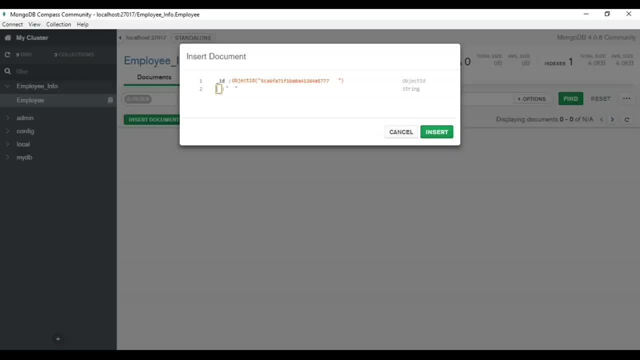 So you can just click on this option of insert document, mention the required values. that is basically the ID dot. object: ID. So basically over here you can just mention employee ID and in this section you can just mention the employee ID. now Similarly you can mention the employee name also. 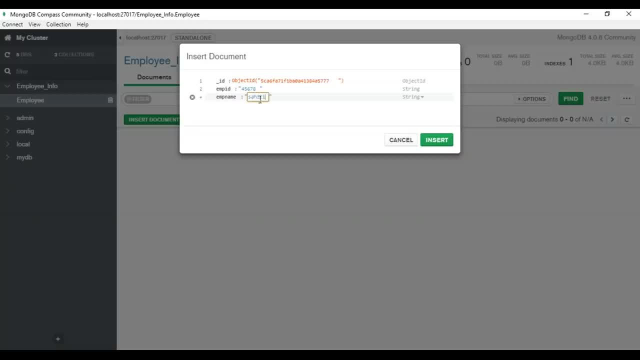 and over here I'll mention the employee name to be, let's say, safety. right now, over here, if you see, we can also use the data type. So let's just say you know our employee ID should be int, So I just mention it to be end and employee name to be string. 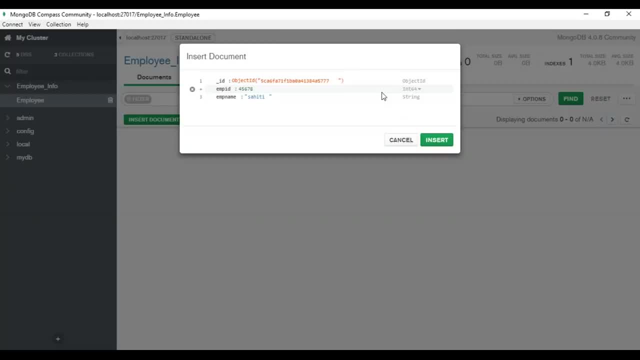 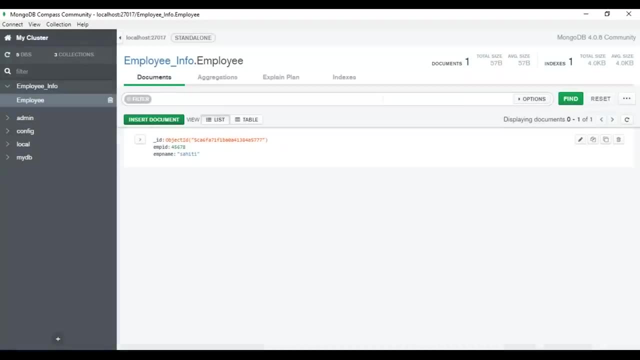 right. So that's how you can mention the data types for your documents And then, once you've inserted all the required values, you can just click on insert. So once you click on insert, you can clearly see that you know your document has been created. now. this you can either view: 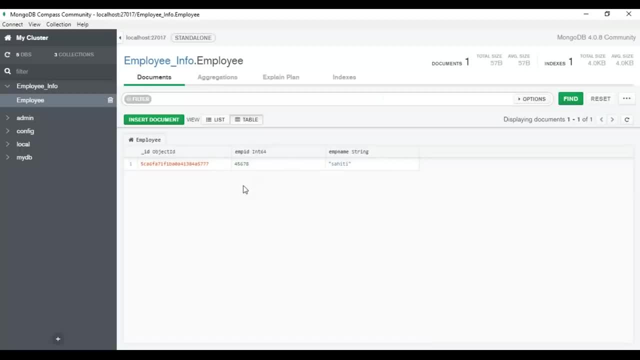 in the form of a table that is basically you know which document ID basically has which employee ID, that is, which data type and also the employee name, or you can also view it as a list. So I was previously viewing it as a list. 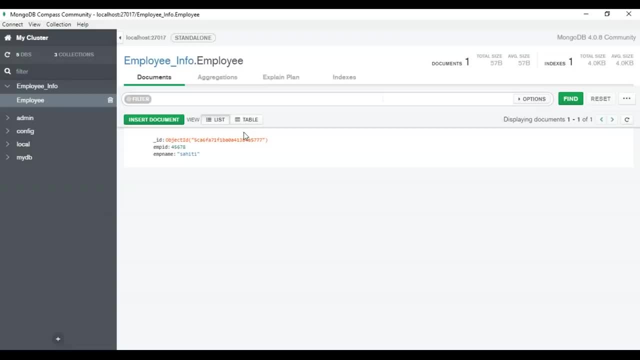 This is how you can create a database and then create a collection and documents. Well, I'm not going to go in depth of how you can use this MongoDB compass and how you can explore much more features of this. so, guys, it was just a short demo on you know. 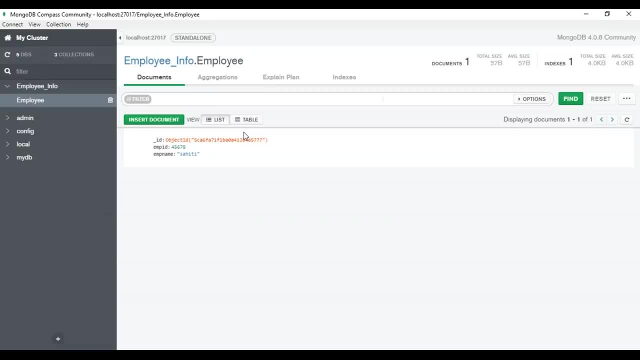 how you can use my sequel workbench and MongoDB compass to handle structured data and unstructured data. So, folks, with this we come to an end of this face-off between my sequel and MongoDB, and I hope you understood all the points now, knowing so much about my sequel and MongoDB. 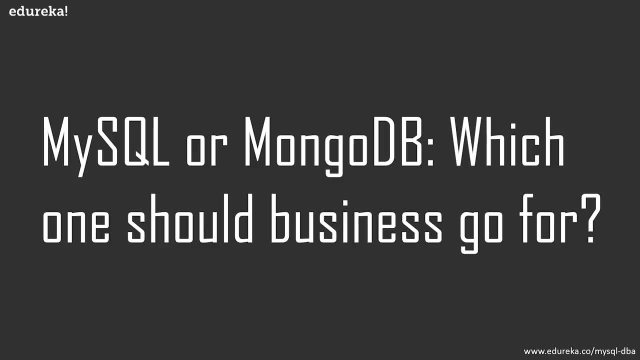 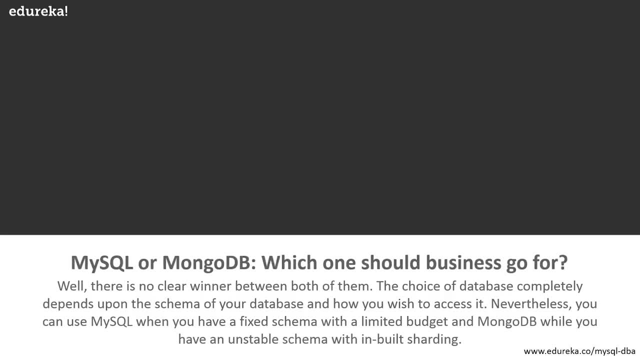 would have definitely raised a question on your mind whether to use MongoDB or my sequel for your businesses. So, guys, well, there is no clear winner between both of them. the choice of database completely depends upon the schema of your database and how you wish to access it. 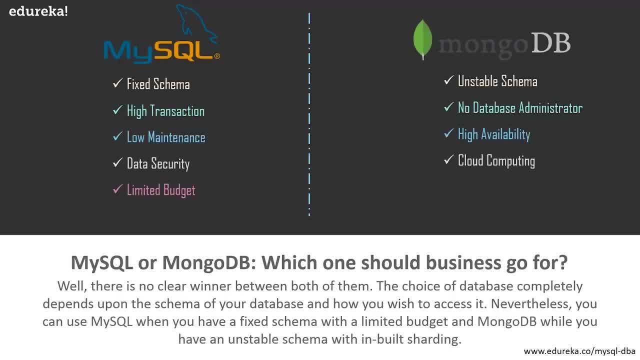 Nevertheless, you can use my sequel when you have a fixed schema, high transaction, low maintenance, data security with a limited budget and MongoDB, while you have an unstable schema, no specific database, administrator, high availability, cloud computing involved with inbuilt sharding. So, guys, this is when you use my sequel and MongoDB.